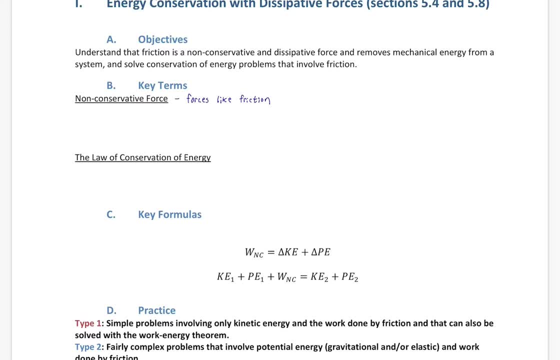 force. you should just think friction. It can also be air resistance or drag or something, but it's always going to kind of operate like friction. Or maybe it's just generally called a non-conservative force, to be more vague. Okay, but what is it? Well, it's any force that removes. 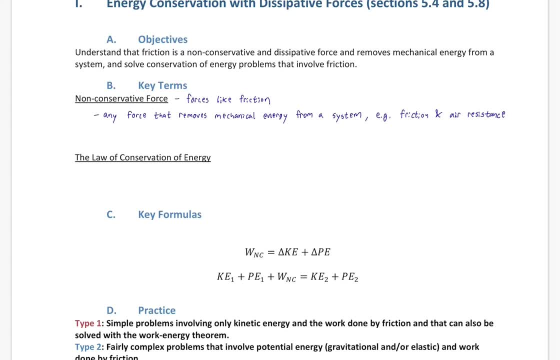 mechanical energy from the system. So we talked about mechanical energy in previous lectures, defined how a mechanical energy is always conserved in an isolated system and how isolated systems don't have friction. Well, now we're going to talk about systems that do have friction, that aren't 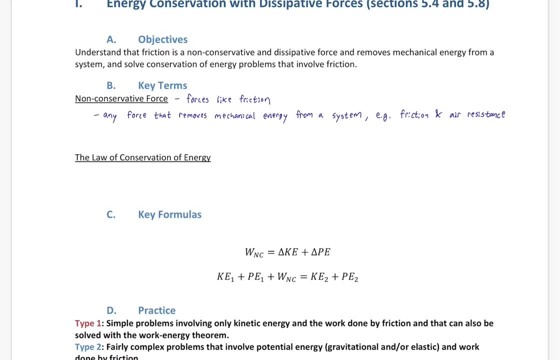 isolated and where mechanical energy is not conserved, And that might seem like, oh, we're just breaking all the rules you know into the story. But actually, as long as we keep things relatively simple, we can use a lot of the same techniques that we used for mechanical energy. 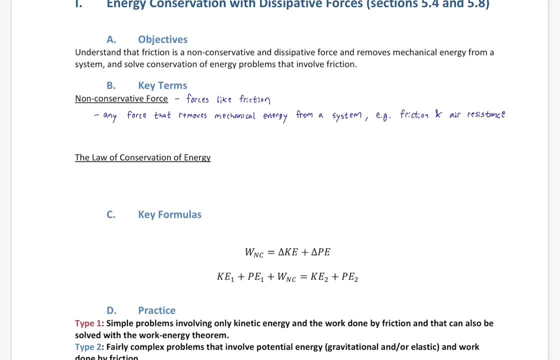 conservation and just account for the friction. As simple as that. All right, we just kind of add one more term. All right? so such a force converts mechanical energy to heat. in most cases, That's where the energy is going. Okay, we're not talking. 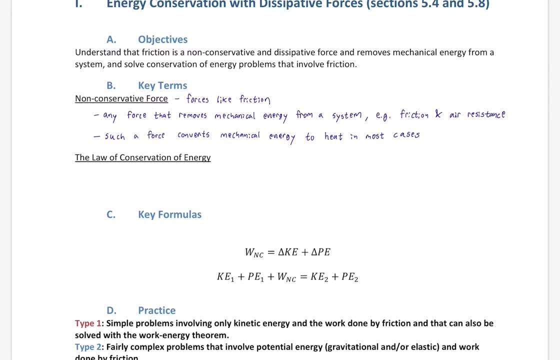 about heat in this chapter yet. but that's kind of foreshadowing things to come. Okay, this also sets the ground, or sets the stage for a big idea called the law of conservation of energy. Notice, this is different than the principle of the conservation of mechanical energy And those 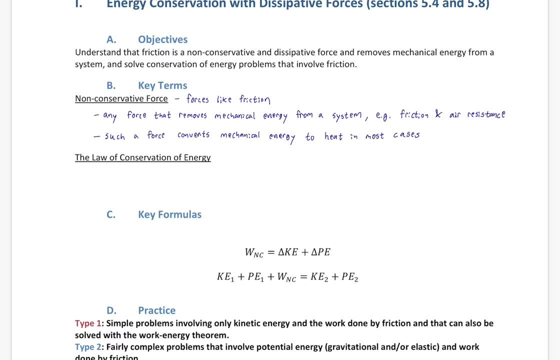 two terms- principle law, kind of interchangeable law- just sounds a little bit more serious. So the law of conservation of energy is one of the three big conservation laws. Okay, we'll talk about that in a little bit, but I won't tell you what they are now. But that's kind of maybe the 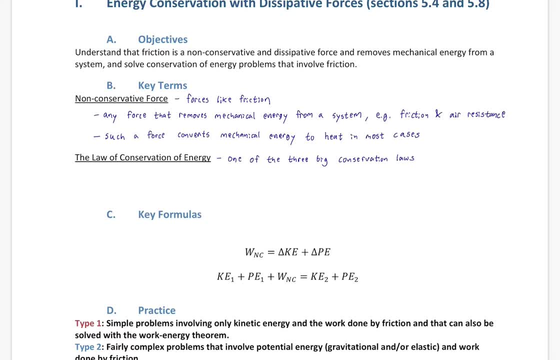 best way to think about it. That was because we really do want to always have those three big conservation laws in mind once we kind of start, once we've got to those chapters. Okay, But for now, what is the law of conservation of energy? Well, it's a general statement that says energy. 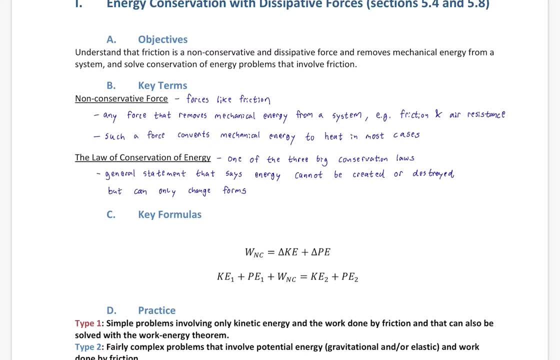 cannot be created or destroyed, but can only change forms. All right, So all those other types of energy that I mentioned in previous lectures that we certainly aren't talking about yet, like electromagnetic energy, heat energy, nuclear energy- Well, it turns out that the 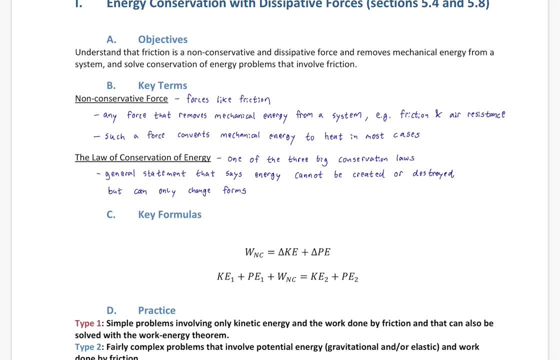 you can have systems where all those types of energy are at play, but they, but no energy is created or destroyed, It's just moving from one type to another. Okay, All right. Nuclear energy can become kinetic energy, even, you know, quite frequently in fact. So I mean that's, that's. 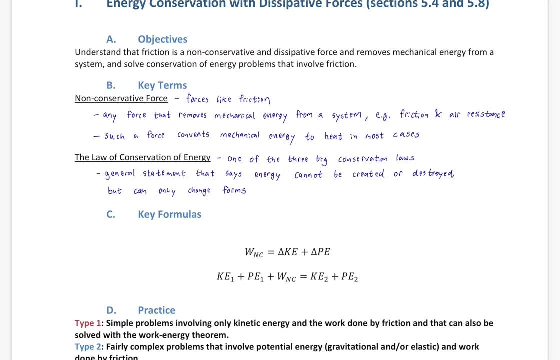 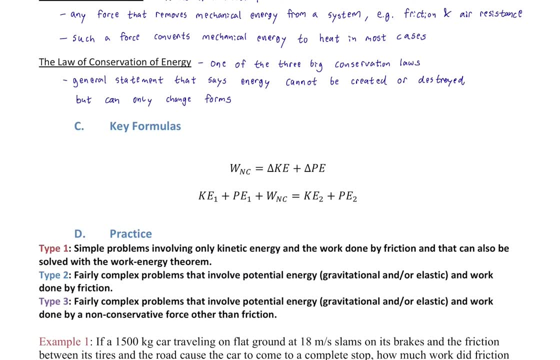 the idea It really cannot be created or destroyed. All right, Okay, Let's get back to talking about mechanical energy plus friction, Cause that's where we're really at content wise. Let me zoom in on these equations a bit, Okay. So this right here is just the way we write work done by a new. 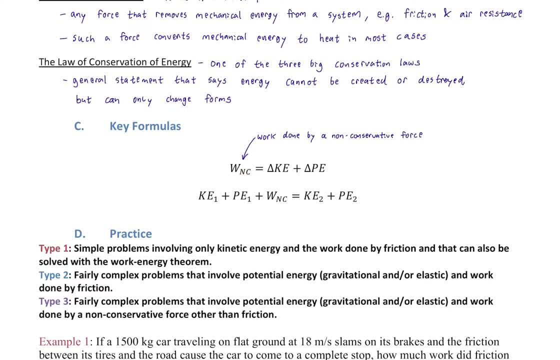 non-conservative force. Subscript. NC stands for non-conservative. All right, And notice what it's equal to. It's equal to a change in kinetic energy plus a change in potential energy. So in other words, we could write it as: the work done by the non-conservative force is equal to a change in. 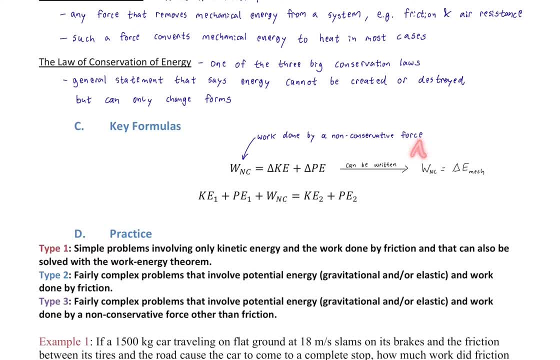 mechanical energy. Cause that's the thing: before mechanical energy was a constant. Okay, It was a constant when the system was an isolated system. but if we introduce a non-isolated system and have a non-conservative force, well, the whole idea is now: mechanical energy can change, but that change. 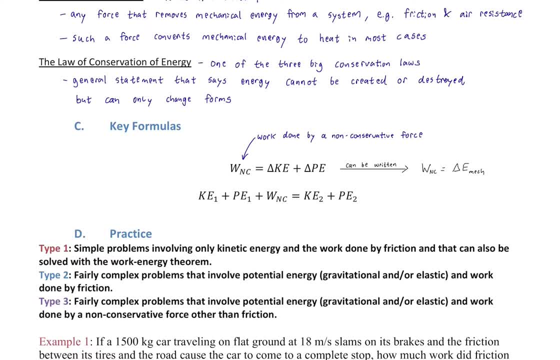 is exactly quantified. It's quantifiable, It's just equal to the work done by the non-conservative force. Now we're assuming a single non-conservative force for our problems, right, Kind of keep you know, keep things you know solvable. in a sense, Okay, And that means that. 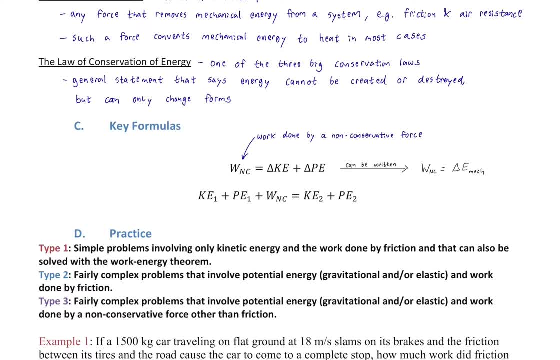 our formula are, you know, kind of E1 equals E2 has an extra term. Check it out. So this, this would be the E1 side of the equation that you know that we solved a lot of problems with. This would be the E2 side over here, And the only thing is on the left-hand side of the equation. 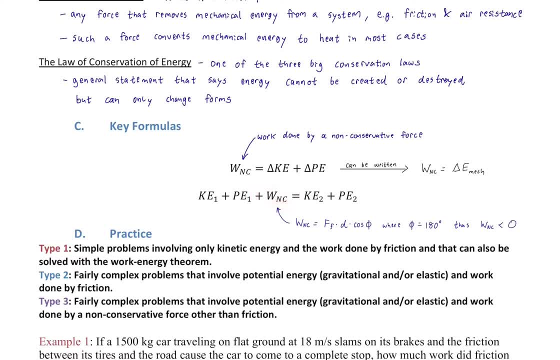 we've added a term, We've added the work done by non-conservative force. Okay, Now a lot of people ask me: why do we add it? Shouldn't we be subtracting it? You know, because I mean. 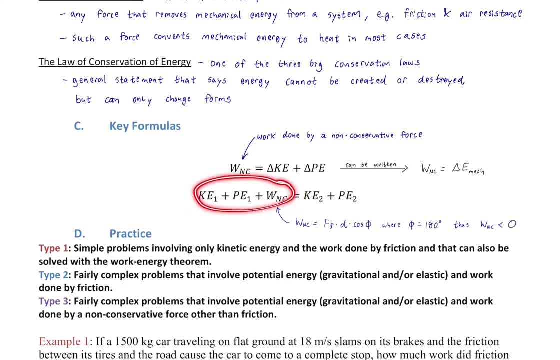 this, essentially, is the energy we start with, the mechanical energy we start with, And if we're adding the work done by non-conservative force, that does that mean that our starting energy is bigger. Shouldn't we subtract it or shouldn't we add it to the final side to say that we have to? 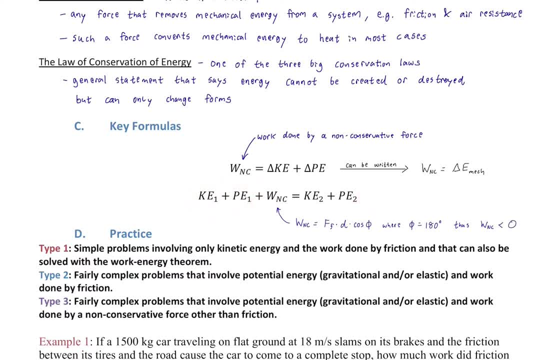 have more energy to start with, because some of it has to go somewhere. Those are valid points If the work done by non-conservative energy is always negative by definition, So you have to add it because you're adding a negative. If you were subtracting it, then you would be double counting. 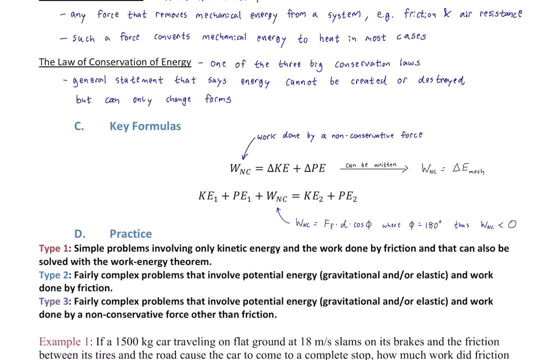 the negative. You subtract the negative, which is like adding, All right, And you might. so then you might ask yourself, or you ask my, ask me, right. So you might say: well, why then? why not just subtract the magnitude? Because we shouldn't, because then we have to remember that we're 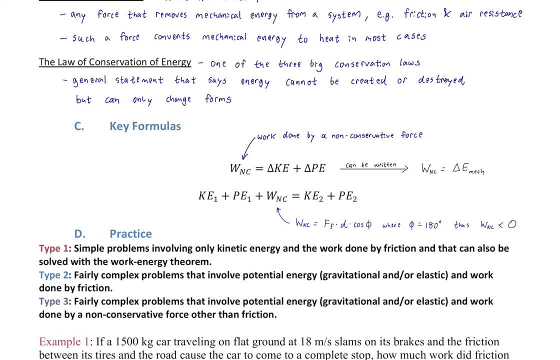 talking about the magnitude, It's better to just stick with the definition of work rather than extra things be like: oh, is this work or is this the magnitude of work? You know that's confusing now, but if we just stick to one rule where we know we always see work and we always know that. 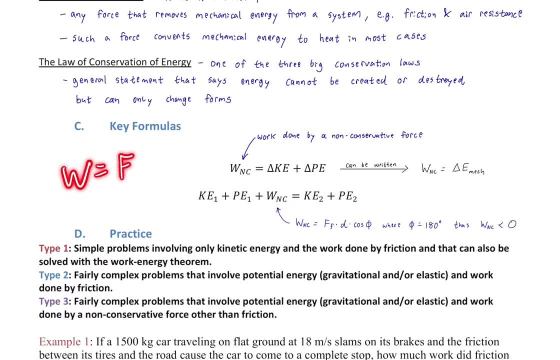 work is always calculated the same way. the definition of work is force times, distance times, cosine of the angle between those two vectors, Then we're we're fine, because that will always apply. All right, And that's what applies here. And that means that when we look, 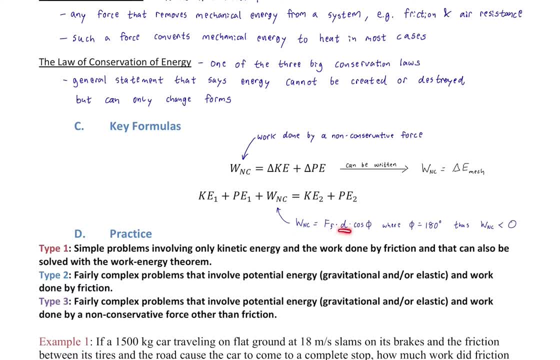 at the work done by the non-conservative force. it is for the friction vector times the displacement vector. There are magnitudes times Cosine of the angle between the two, And the angle between the two is always, always, always, 180 degrees. Friction and air resistance, otherwise known as drag, always oppose motion. 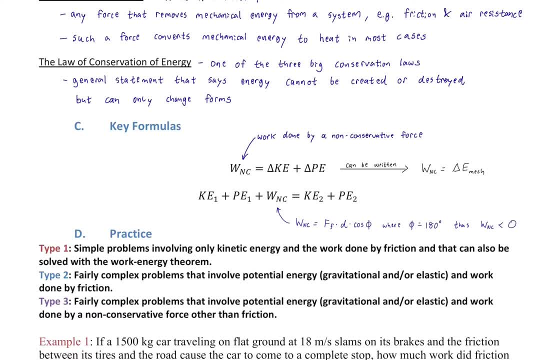 They always oppose the velocity. That's that's what they are, And since those are the only type of non-conservative forces that we're going to see, that means this angle is always 180, which means that the work done by non-conservative forces is always less than zero. It's always negative. 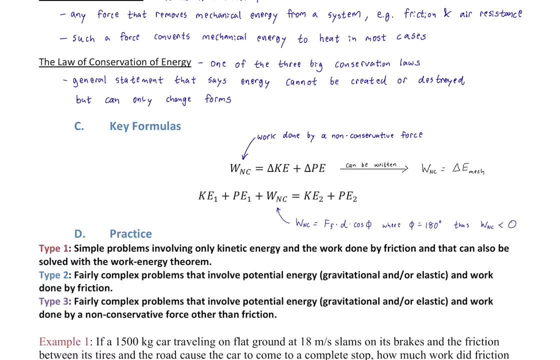 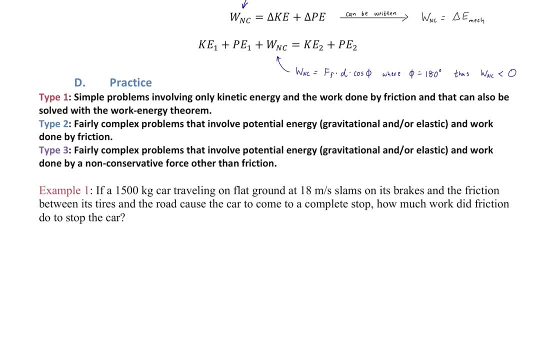 which is why we have to add it. Okay, All right, Get the point. Let's do some examples, All right? So type one: simple problems involving only kinetic energy and the work done by friction, and that can also be solved with the work energy theorem, All right. Type two: fairly complex, 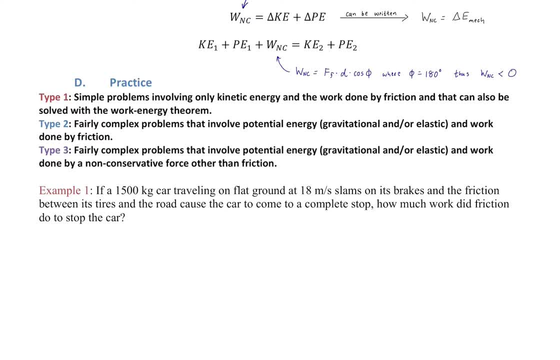 problems that involve potential energy, gravitational and or elastic, and work done by friction, All right, So that those ones couldn't be really easily solved by the work energy principle, because we've got, if we have a spring in there, we can't really express the work done by a spring. 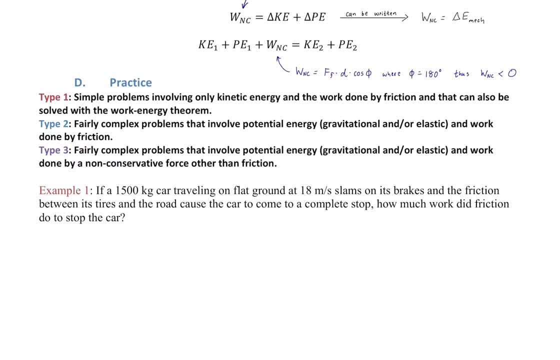 unless we use an integral and we don't use calculus in this class. So in that sense we kind of we kind of have to use the whole energy conservation equation. but it's a fine line, All right. The point is that they're a little bit more complex. Okay, And finally type three, fairly 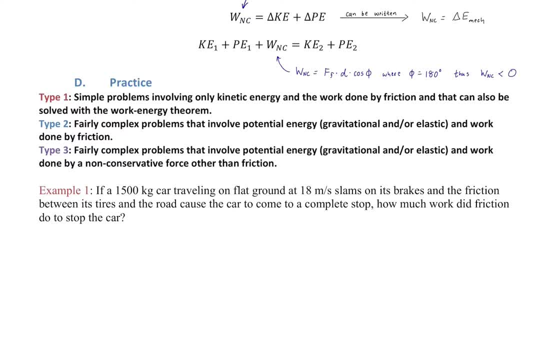 complex problems that involve potential, energy, gravitational and or elastic. elastic and work done by non-conservative forces other than friction. Okay, So that would just be basically drag or air resistance. All right, So let's look at the first one. If a 1500 kilogram car traveling 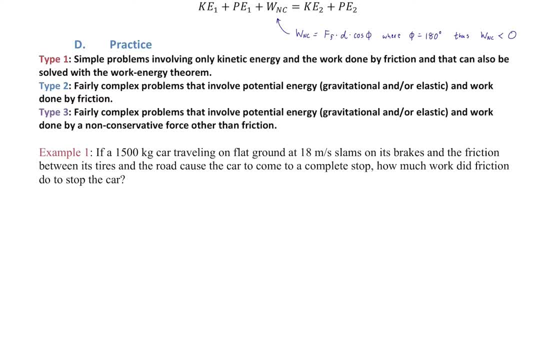 on flat ground at 18 meters per second, slams on its brakes and the friction between its tires in the road caused the car to stop. then how much work did friction do? All right, Well, that's definitely one that we kind of. that we would have seen back in the definition of work. 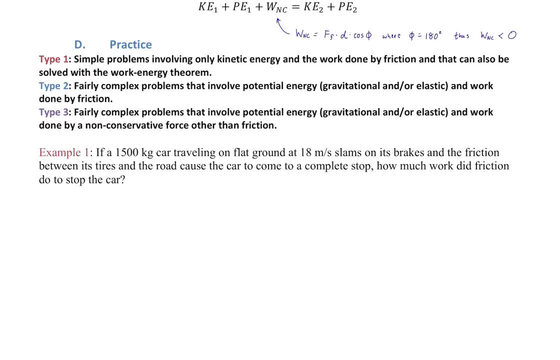 chapter because we could just say: oh well, it's just work equals kinetic energy, All right. So we could definitely solve that: the work energy principle. If we set it up this way, using our new equation, E1 plus WNC equals E2, then E2 is zero because the final state is no. 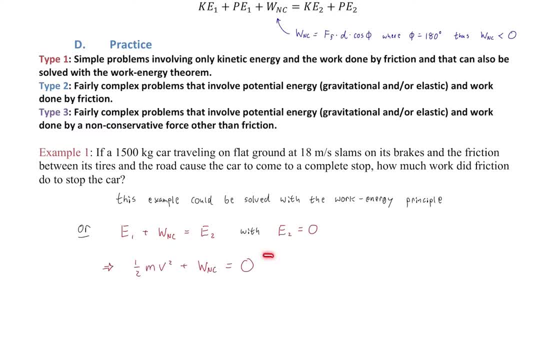 energy. There's no kinetic, no potential, And so then our formula just becomes this: and then we're going to solve for the work done by non-conservative forces, which has, which we see, naturally becomes negative. Okay, As it should. Okay, And then plug in our numbers and we have. 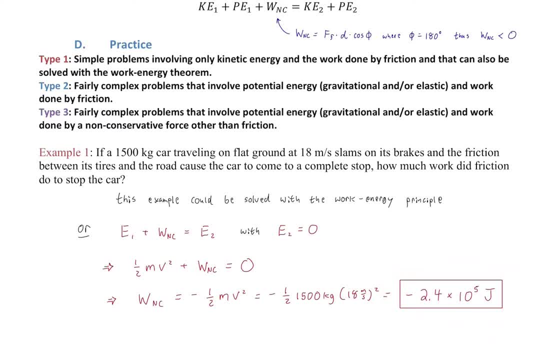 negative 240,000 joules. right, That's how much work friction does. Okay, That's how much energy friction removes from the mechanical system. Okay, All right, cool, Let's do it again. So this one. I actually forgot to give you a piece of information. Um, when you, when I give you, 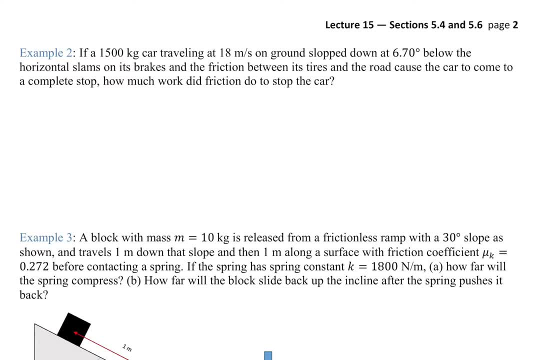 a problem like this and notice it's very similar to example one. but now there's the cars either going downhill or uphill. I have to either give you the friction coefficient if it's a constant slope hill or I have to give you like the length of the hill. So here what I should have given you. 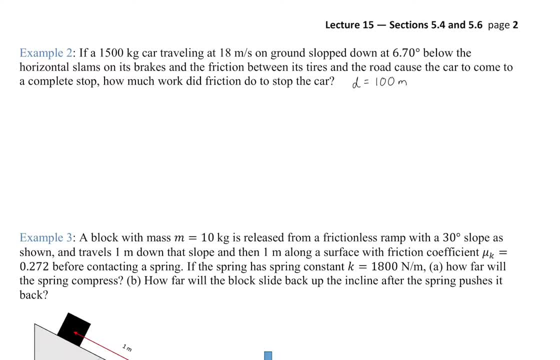 is the length of the hill Cause. otherwise you don't have enough information to solve it because it depends, Does it? basically? friction will do more or less work, depending on if friction acts really quickly and stops the car really abruptly or if it stops the car really gradually. Okay, 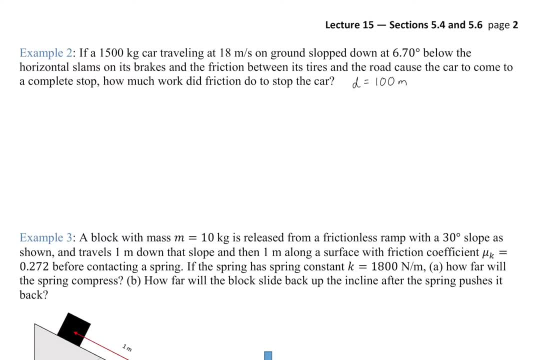 And it's, and it's just, it's just a function of that effect. All right, Cause the idea. if you look at the picture here, the car's going downhill So you think about it. friction acts really fast. then there's almost no change in gravitational. 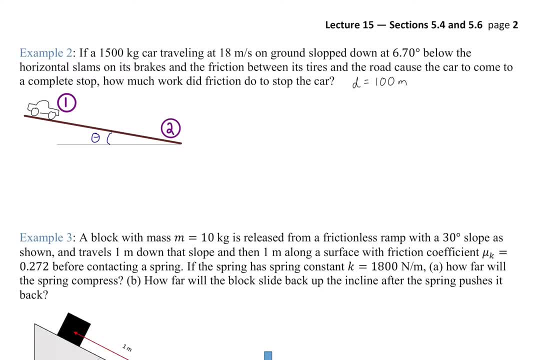 potential energy, All right. But if friction acts really slowly, then there's actually the car lost energy, lost gravitational potential energy, And so then the friction has to deal with that extra loss of gravitational potential energy that then became kinetic energy. All right, So there's a 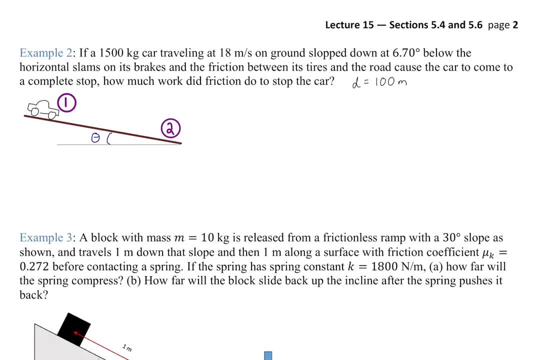 there's a real difference here between between how how the friction is going to act. Okay, So with a hundred meters that means it does go a ways downhill, and we're going to use. E1 plus the work done by non-conservative forces equals E2.. We'll define E2 as zero again. 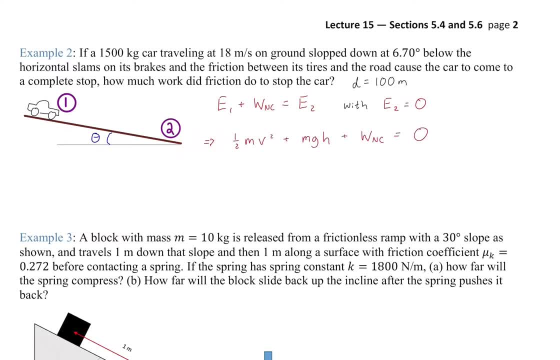 because since we're we're saying the bottom of the hill is y equals zero. All right, So then our E1 is the initial kinetic energy. The initial gravitational potential energy is that MGH. H would just be this height here, Okay, And then we have the work done by non-conservative forces. 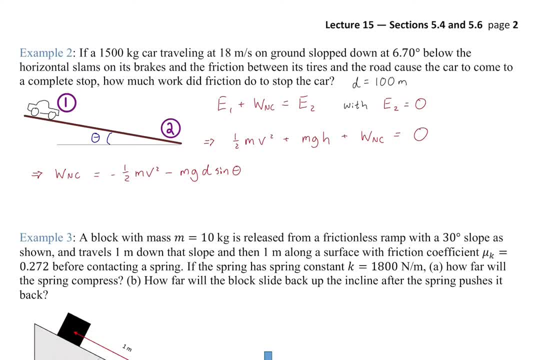 All right, Then we're just going to solve for the work done by non-conservative forces. Notice my H becomes D sine theta right, Cause D is this distance. Okay, And so H is just this side of that right triangle. All right, And then we plug in all. 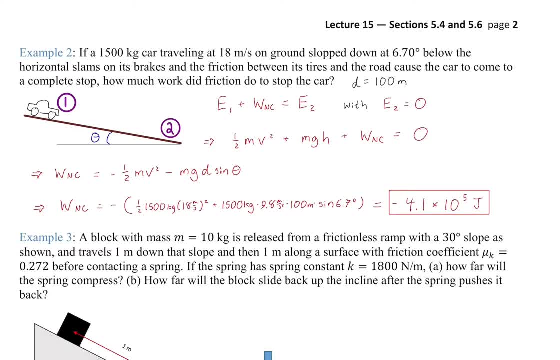 our values and we find that in this case, friction does negative 410,000 joules. And notice, this was the same car, All right, Traveling at the same speed, But the fact that the car was going downhill meant that friction had to do a lot more work. 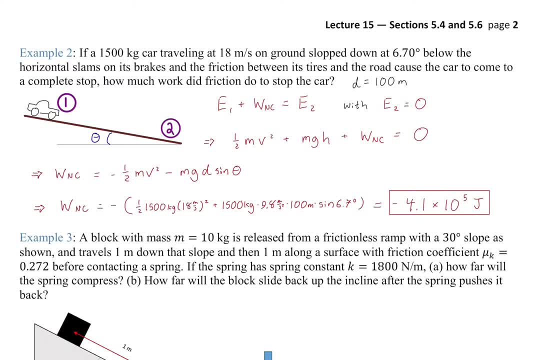 not more negative work, right, It had to remove a lot more energy, And that makes sense, right, Because it on the level ground friction didn't have to, you know, deal with the extra kinetic energy that gravity was creating. but on the downward slope to ground it does have to deal. 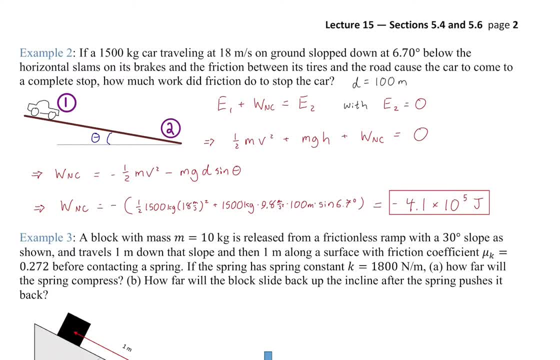 with that extra energy, All right. So that means more work is required from friction. If it was going uphill it would be less right. Okay, Cause then essentially the hill is helping out friction in terms of getting rid of the kinetic energy Friction has, then is able to do less work, All right, And that's one of the 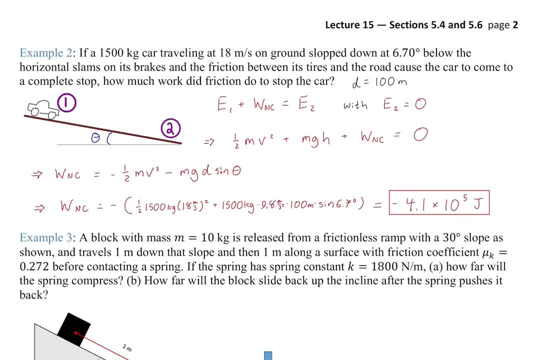 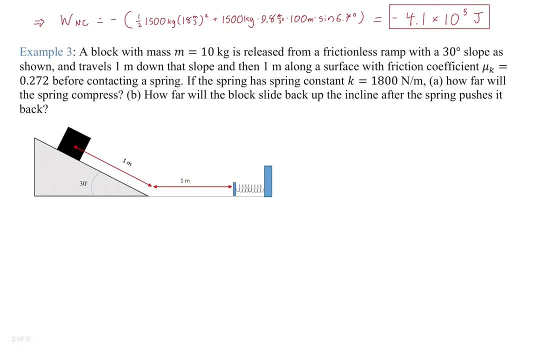 questions I asked. in the kind of the follow-up examples We have the car going uphill, but that time I give you the friction coefficient to mix things up a bit. All right, Another example: a block with a mass of 10 kilograms is released from a frictionless ramp, So we got no friction. 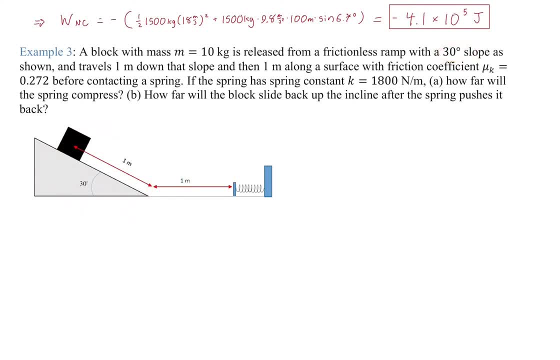 in this part. Okay, 30 degree slope, Um, and we? if you've watched previous lecture videos, you've seen the same problem, but a frictionless one. But now where's the friction? come in? It comes in on the ground. So this whole section down here. 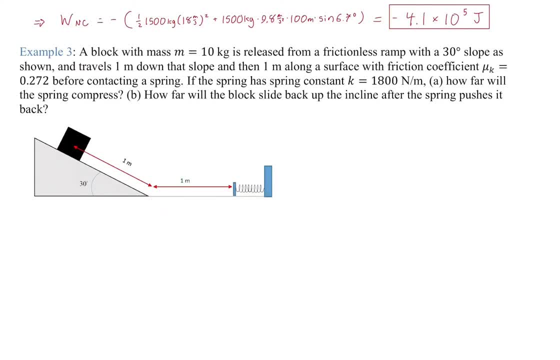 has friction and it has a friction coefficient, a kinetic friction coefficient of 0.272 kinetic, because the block will already be in motion once it gets down to the ground. All right, If the spring has a spring constant of 1800 Newtons per meter. 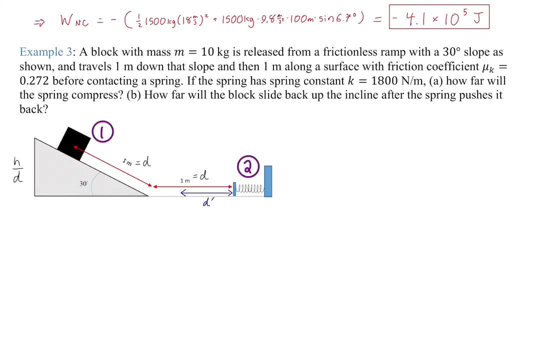 then question a: how far will the spring compress? Okay, We can definitely do that. We'll set up our two states, state one and state two. We're going to call those two distances- The one meter distance is D, just so we can kind of keep it symbolic and clean for a while and plug. 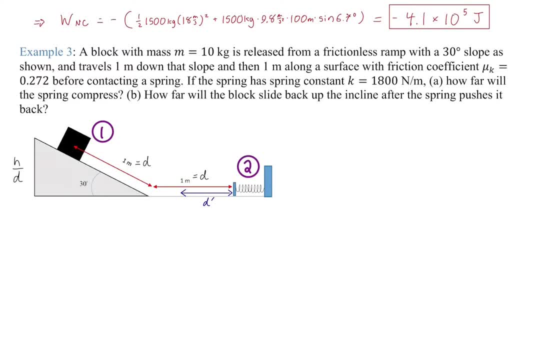 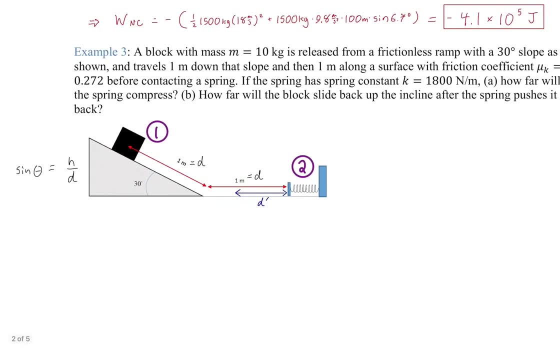 in numbers at one step, All right. I always think that's a better way of doing this kind of work. Um, and then here we just have um, uh, H over D. Oh, there it is. Sign of theta equals H over D. 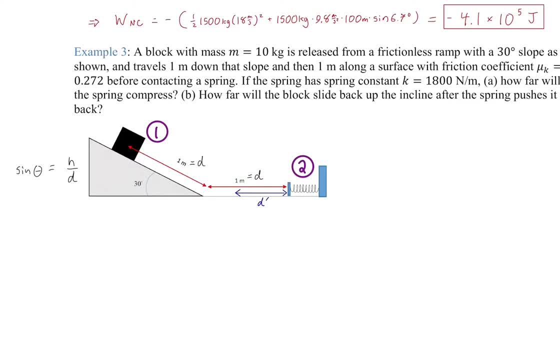 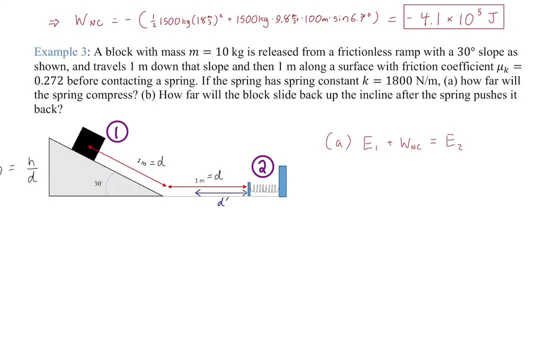 And this will allow us to solve for H in terms of D. Excuse me, Okay, All right, So moving on. uh, we have our energy conservation right. This is our new new form. right For this lecture. right, It's always going to be E1 plus work NC. 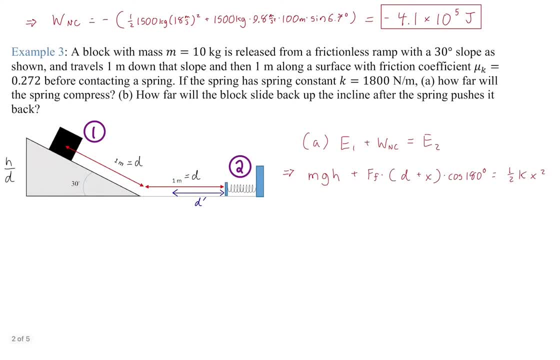 two. Okay, So what do we know? Well, we know we start with some gravitational potential energy, MGH We're going to have. the friction is going to be D plus X. So D is that, that, that fixed distance, We know? the friction acts over it And then X is just going to. 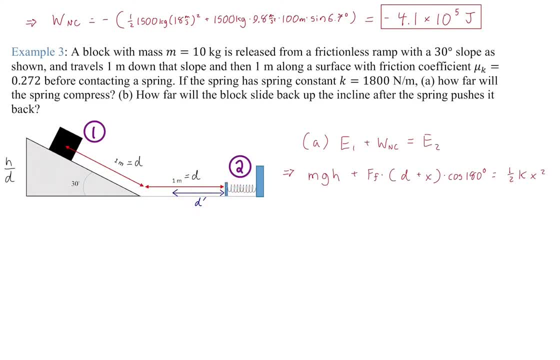 be the compression distance. Don't worry about that D prime, that's in part B. So X is just going to be this distance here. That's X Okay, Because the friction will continue to act as the spring is compressed, because after all it is the same surface. 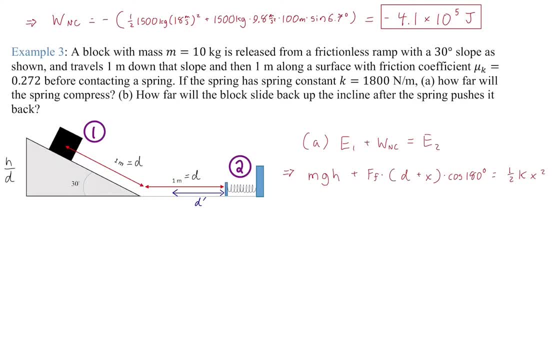 It's not like the friction magically stops acting, You know, when the when it reaches the spring. now we could have a change in surface here and we could define it as such, but I think it's more natural to say: well, this is all the same table. 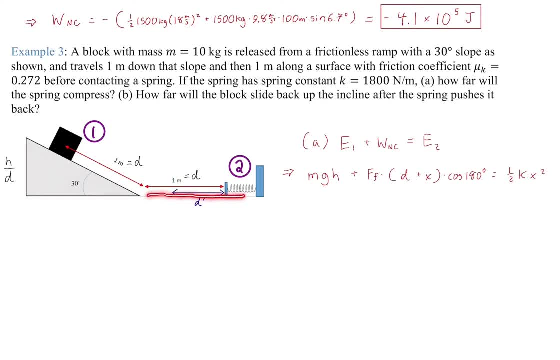 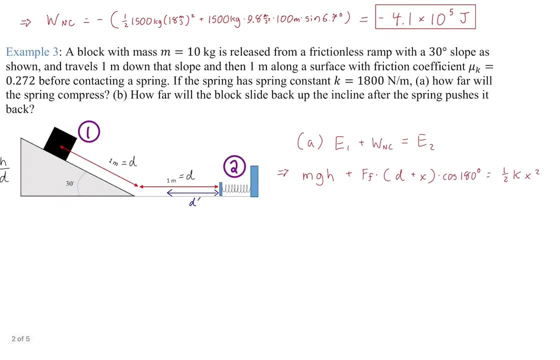 right, You know, if we're actually built this thing, And so friction would have to continue the whole way. All right? Um, we have cosine of 180 degrees, which is just going to make this term negative. Okay, And then the final energy E2 is the, the, um, elastic, uh potential. 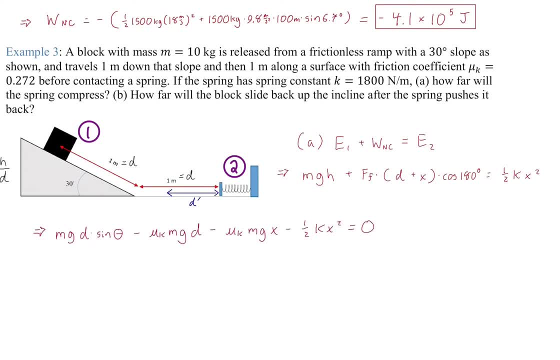 energy of the spring. Okay, Because the spring is storing that energy with the energy that's left over that didn't get converted. the heat from friction, All right. So there's our gravity, our initial gravitational energy. here is friction, um doing its work on the one meter stretch. 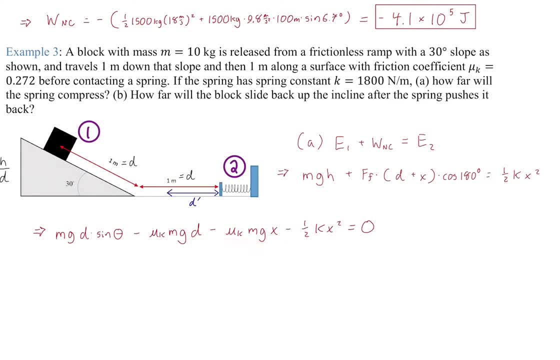 which we call D. and here's the friction doing, continuing to do work over the compression addition distance X. And here is the gravitational um stored energy. All right, Excuse me, the elastic stored energy which I just moved to the left-hand side So I could set the whole thing. 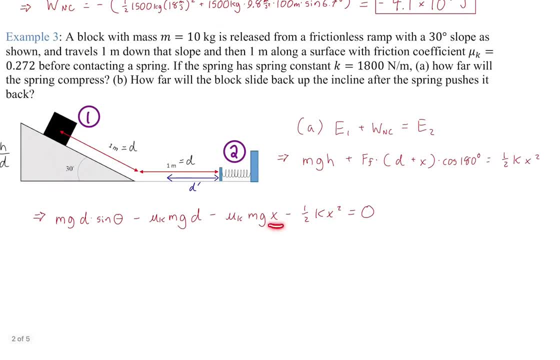 equal to zero. Why do I want to set the whole thing equal to zero? Well, because we have an X and X squared and we're solving for X, right? So I want to make this look like you know, a second order polynomial, So I can use the quadratic formula or, in this case, I'm just unplugging. 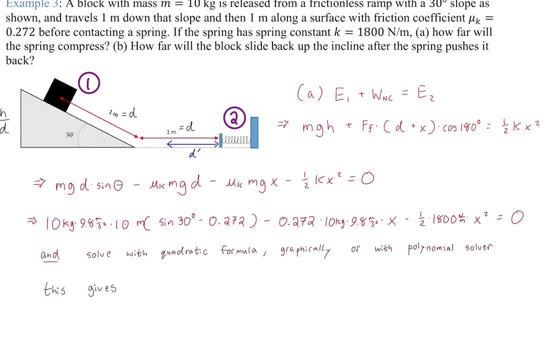 all my numbers and then either graph it um use a quadratic formula or solve it with a polynomial solver which is built into. you know, calculators like like Desmos, or you can ask Google to do it, or the Texas instruments have built in polynomial solvers And when we do that we get a value of. 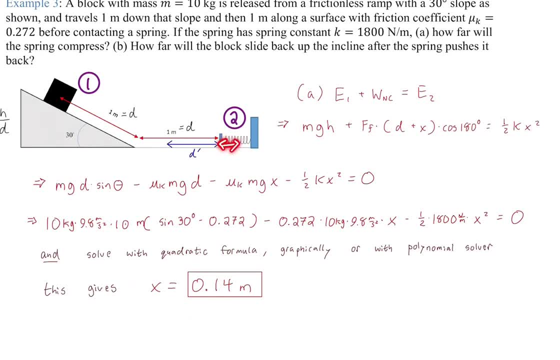 0.14.. So the compression distance of the spring is 0.14.. And if you consider the same problem with the same block and the same amount of gravitational potential energy, when it's friction, frictionless, the compression was, I think, over 30 centimeters. So friction has done a significant amount of work. 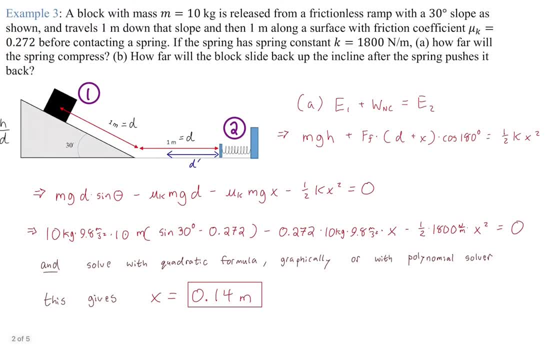 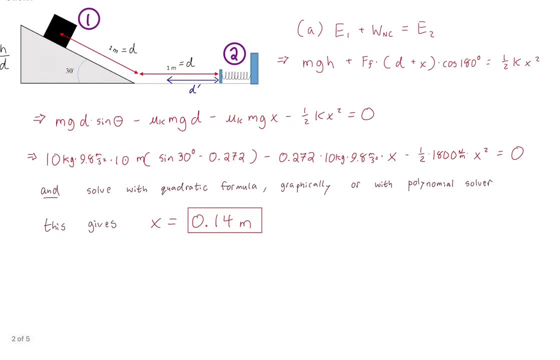 here, Um, but that's because it's a fair. you know, it's a fairly small block, which means it didn't have that much gravitational potential energy And the friction coefficient is fairly large. Okay, Especially for a kinetic friction coefficient, All right. So that's part A All. 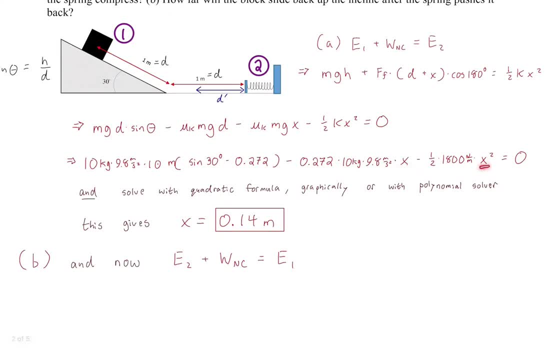 right, And that that one was tricky in a sense, because you know we had, we had to solve for X, where we had an X, X and an X squared, All right, But what about part two, or part B, That is, I say, 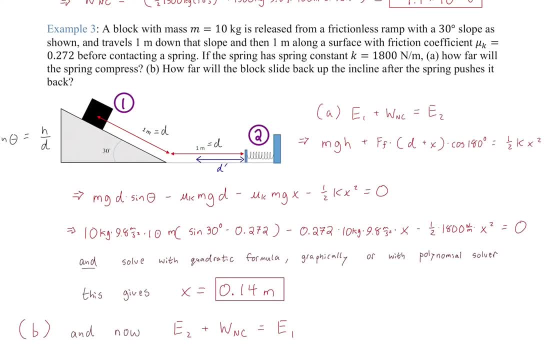 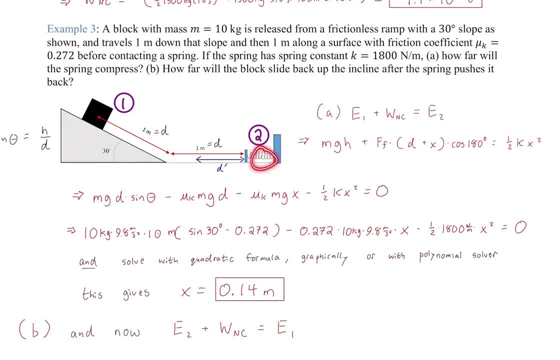 well, what do we? what energy are we going to start with? Well, we're going to start with the stored elastic energy, All right. And then we're going to. friction is going to start doing work again as the block starts to travel back this way. And then we just wanted to find out, you know how. 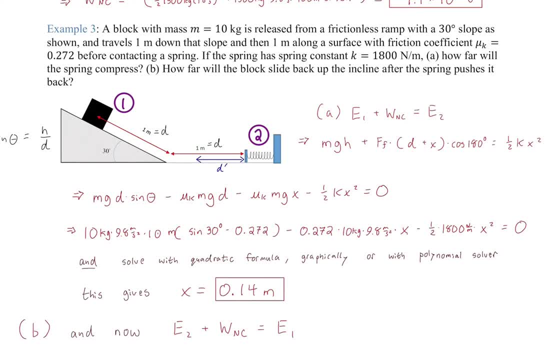 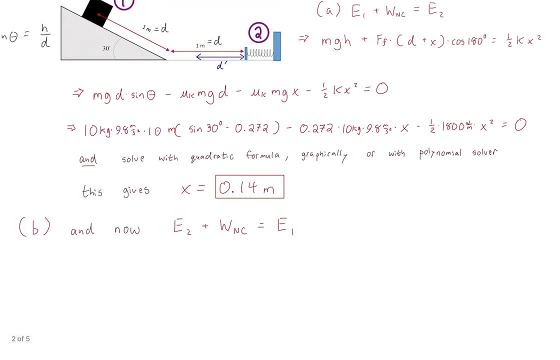 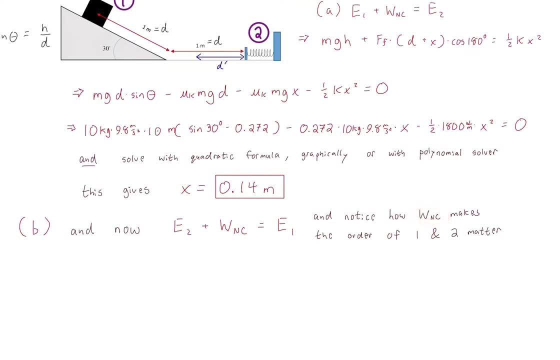 I put a note here and notice how the work of non-conservative force makes the order of one and two matter. What I mean by that is because I even mentioned this when we were dealing with just mechanical energy without friction, And that's the previous lecture, by the way, that would be. 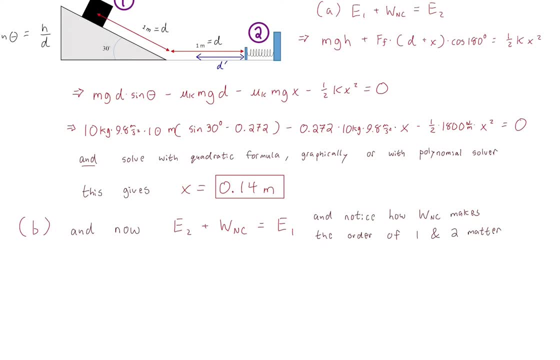 lecture, lecture 14, that when we were, when we were doing that, we didn't really we didn't have to worry about, you know, whether we were going from one to two or two to one, because it was the same, It was totally interchangeable, And and that's, that's because you know the gravity is. 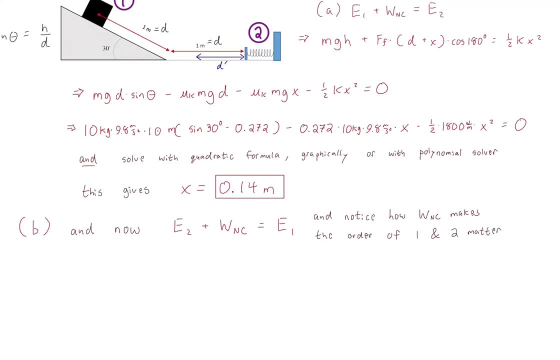 this thing called path independent. It doesn't matter how you get there, It just matters You get there. The kinetic energy is going to get converted to gravity or gravity will get converted to connect energy, And that just. they're totally interchangeable. but once you have friction, 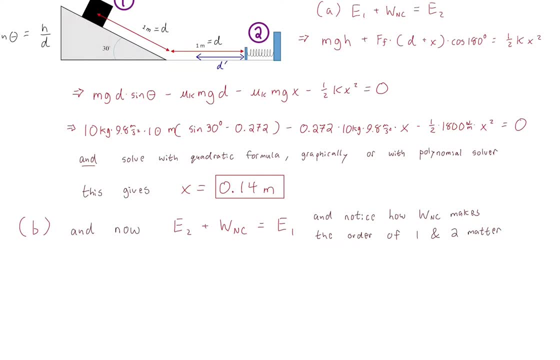 they're not right, Cause friction just continues to take away energy. All right, Friction friction did work on the way down. It's going to do work with continue on the way back up. All right, So you can't it that. you'll see on the final. 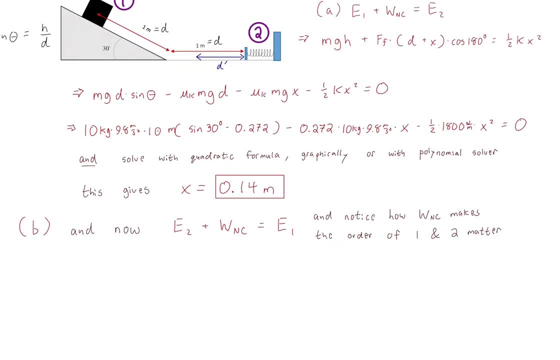 example of this lecture. that means that you can't like skip a point, because before, remember, I said: well, you can, and the best example is a concept question where we had we went from, you know, 0.1 to 0.2,, or we went from 0.2 to 0.3, or just jumped from 0.1 to 0.3.. All right, It was. 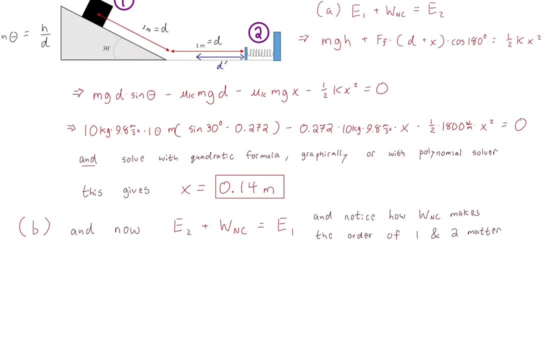 a concept question of dropping the block on the spring. Please refer back to lecture 14 and see the concept question of dropping a block onto a spring and filling in the table of whether the changes in energy were positive or negative. And we could totally just skip over 0.2.. You can't. 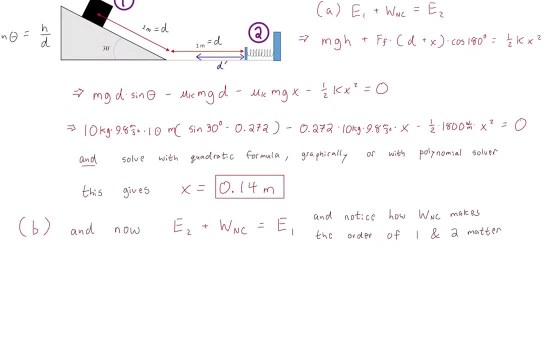 skip over 0.2 when you're doing friction, All right, And so essentially we could call- we could call this three right, Because really it's actually a different energy state, but I'm kind of. I'm kind of calling it one because 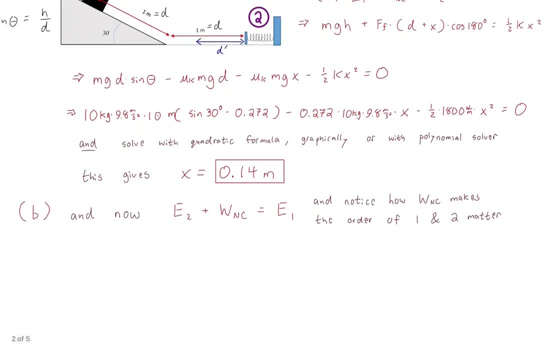 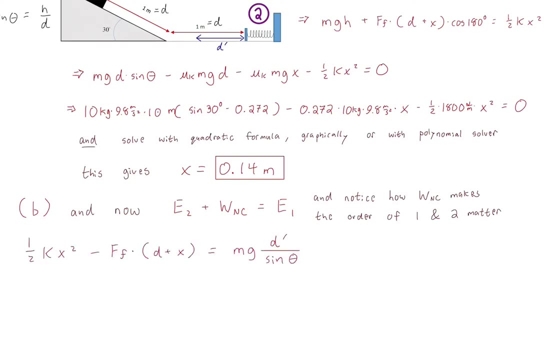 I'm hearkening back to you know, getting back up to some height on the map, but we'll turn out what turns out, that it never gets it back. It never makes it back to the ramp. Let's see, Right, And it's kind of cool because we don't have to, we don't have to assume that we can. 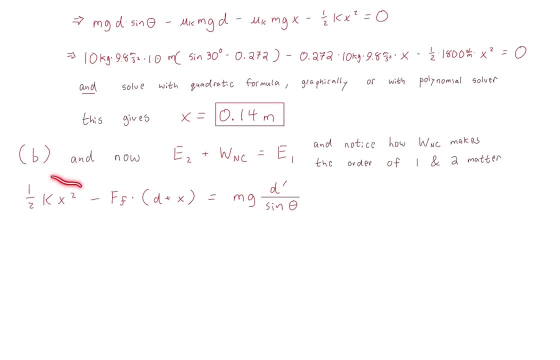 just find it out, but I'm getting ahead of myself. Check it out. Okay, So here is the initial stored elastic potential energy. All right, Here is the work that being done by friction. it's negative And I'm not showing why this time, but obviously it's because it's. 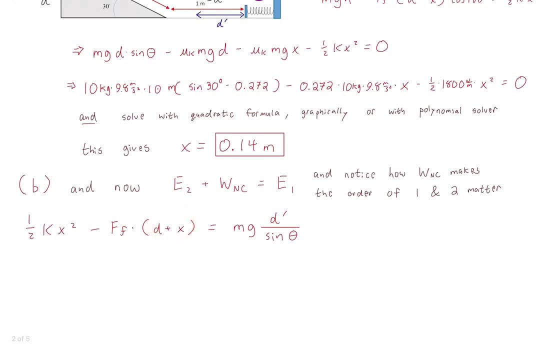 cosine 180.. All right, And it's going to be D plus X. Okay, We know, we know what X is. We'll use the X we saw for, because that is the correct X, The D, I'm assuming it's going to travel the. 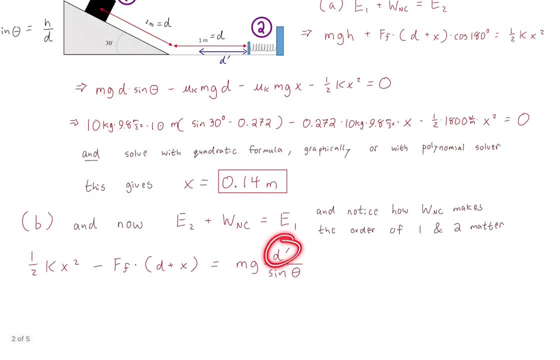 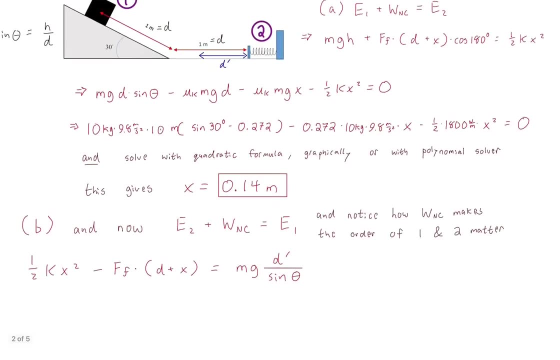 whole distance back to the ramp. That's the point, Right. And then my D prime here is going to represent how, how high it goes up the ramp. Okay, All right. So then, and then you know, D prime is just going to be, you know from from this, this relationship here, it's just going to. 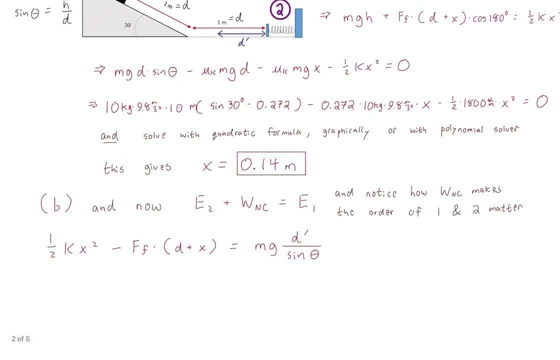 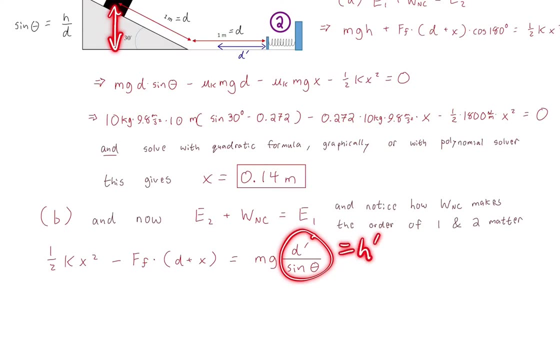 be H over sine theta. Okay, Okay, Or I guess really what I'm doing is I'm solving for H prime, because initial H is this And so this right here would represent H prime, the new height, right, How far it makes it back up the. 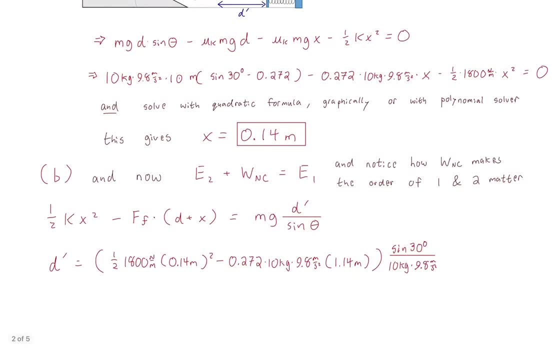 ramp. Okay, So I set this all up. Don't have to worry about the quadratic formula here, because it's I'm just solving. I'm just solving for the one unknown. All right, Plug in all my numbers, But I get a negative. What does that mean? Shouldn't D, shouldn't I mean, after all? 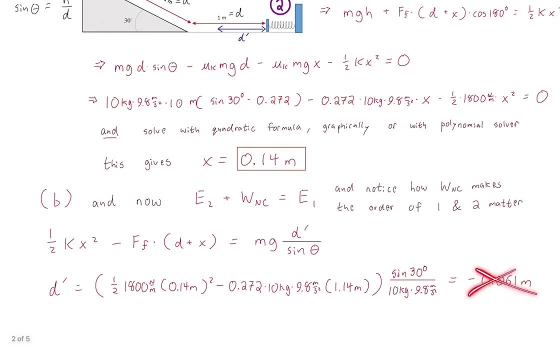 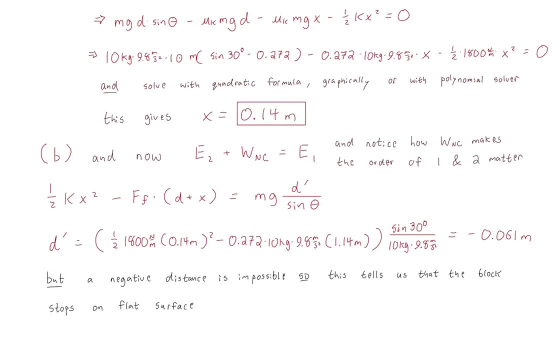 you know, D prime is a is a distance. A negative distance has no physical meaning. Okay, That's not right. What happened? Did I make an error? No, But there was an assumption that was off. Okay, But a negative distance is impossible. So this: 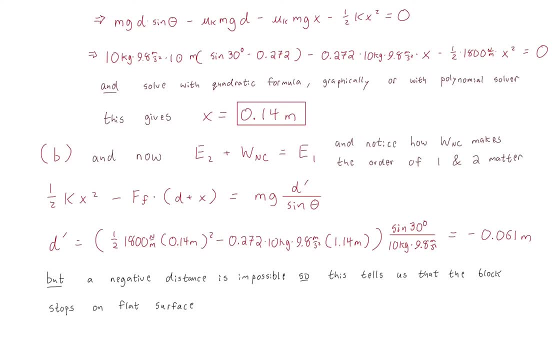 tells us that the block stops on the flat surface. So I love problems like this where you just say, okay, I'm just going to, you know, set something up and solve for it. Right, It's totally valid to ask for how high it makes up the ramp, But then I get an answer that makes no physical sense. 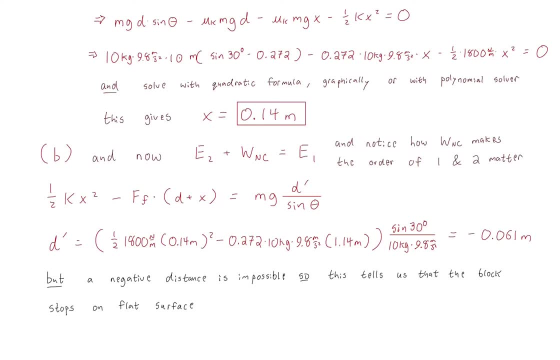 That's because the question was, yeah sure, A trick question, but it was a good. it was a good trick question because it was like it was a valid question to ask, Right. And so this, this answer, although it doesn't make physical sense, tells us a very direct thing. It tells us that we have to 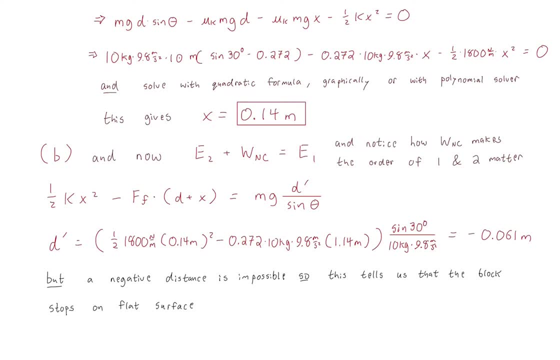 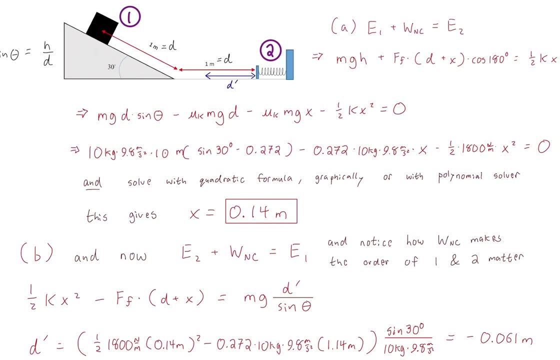 change our conservation of energy equation and don't include any gain in gravitational potential energy, but instead solve for a D prime that is along the flat part. Okay, So what does that look like? All right, So that will just look like this. So this is just the stored elastic energy Here. 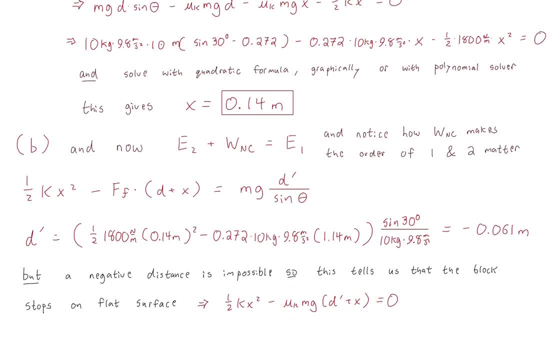 is friction doing its work And notice that that's, there's no other term, because E2 is zero. now, because it's going to, it's going to stop on the flat ground, So it's not going to have any gravitational potential energy to end with. All right, And so then I'm just going to solve for D. 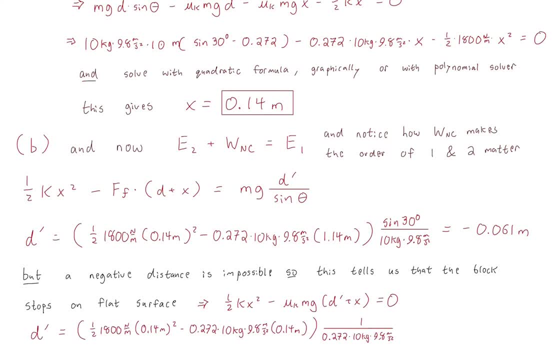 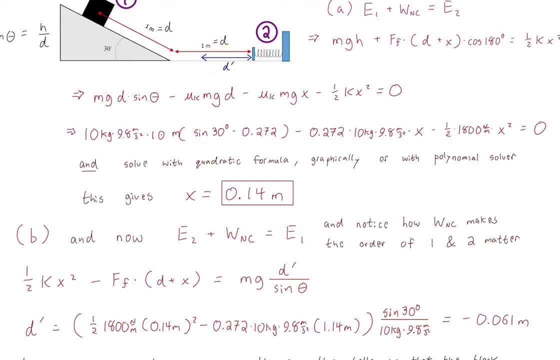 prime And when I go ahead and solve for D prime, but plugging in all the numbers I get 0.55.. So that means that it stops somewhere right around here. It makes it about halfway back to the ramp and that's it. And again cause there's a lot of friction here and it just come to rest, never to. 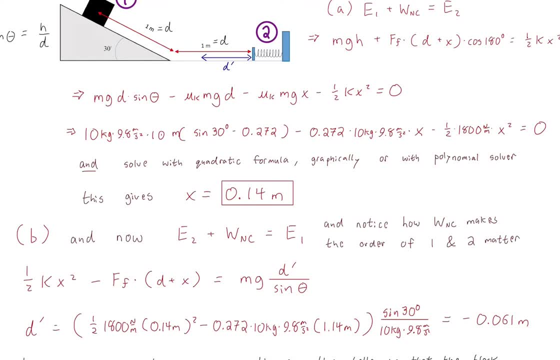 move again. Okay, So that I mean I that's what's cool about these, these friction systems, is you can kind of actually kind of continue them until they could. they stop completely until friction has removed all the energy. So that's, that's, that's, that's, that's that's. 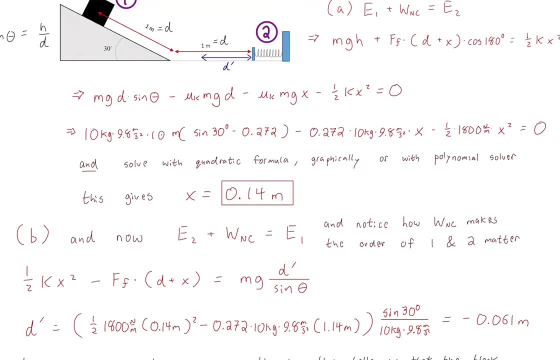 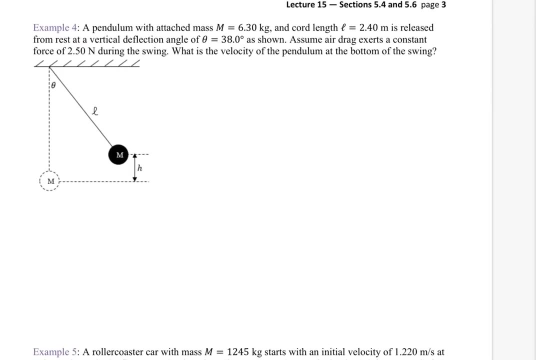 all the mechanical energy from the system, All right, Even when there's a kind of, there's a back and forth, a storing, a storing of energy in the spring in this case. Okay, All right, Let's do another one. Here we have the pendulum, All right, So pendulum, pendulums are great systems. 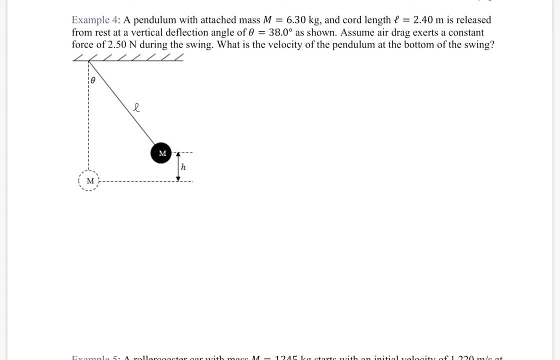 for um, for mechanical energy, because you can't do Newton's laws with them. I mentioned that before. I think it really highlights one of the utilities of using conservation of energy equations. but pendulums can also have friction. Now we have to be careful with how we're going. 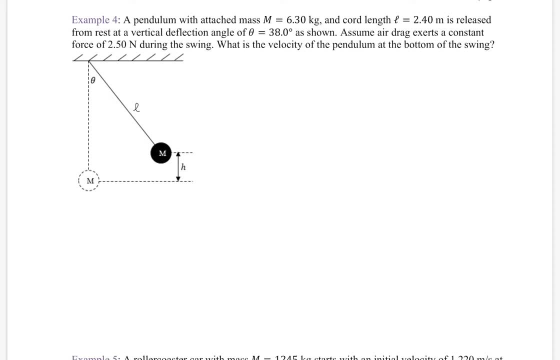 to do friction. We can't do it in a very realistic way with the pendulum. So instead, I'm just going to say that there is a, an average force, which is a constant force that's exerted by air drag, And I'm just going to give it a value. So essentially, there's, you know, there's this. 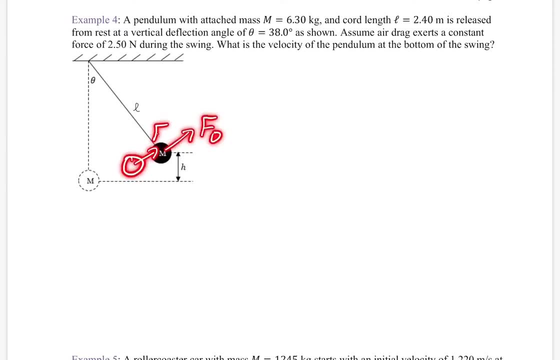 drag force exerted on the, on the pendulum Bob, at any given point as it moves in its path. Okay, And that value is always 2.5 Newton's. That isn't that realistic. The first, the um drag forces. 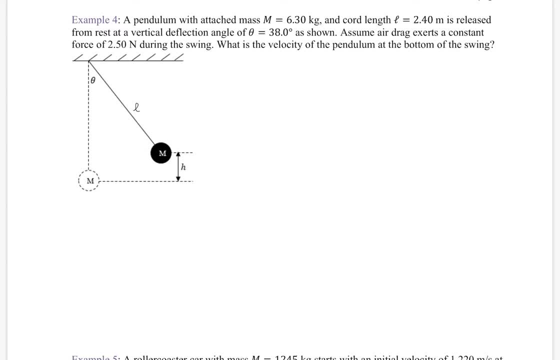 are always proportional to velocity And um. but you know, we can kind of just simplify it here and say: okay, it's just 2.5 Newton's, Okay. So let's set this up: We have 0.1,, we have 0.2,. 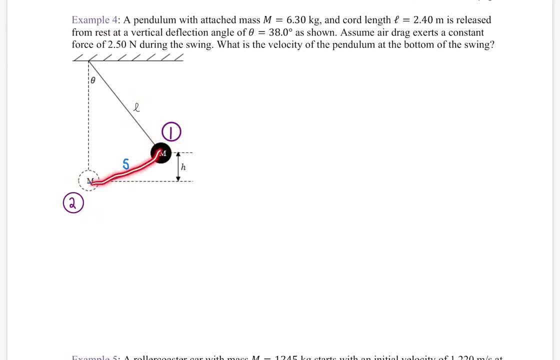 the length of the pendulum string is L, And then we got this thing, S, which is the arc length. How are we going to find that? Okay, Well, first of all, we were definitely going to start with the same equation: E1 plus the work done by non-conservative forces equals E2.. All right, 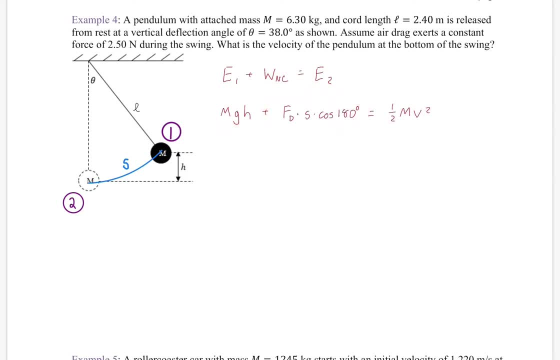 So we start with gravitational potential energy. Here's going to be, here's the friction. It's going to become negative because that cosine 180, and here's the final energy, which is all kinetic. Okay, And then what's that S? Well, S is the path length, and we can find it as a ratio of the. 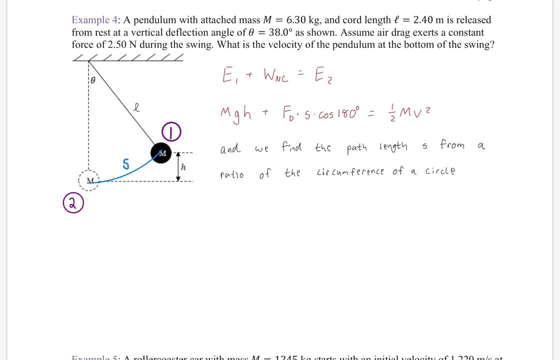 circumference of a circle. All right, So it's the path length. It's also called the arc length. Simply, the ratio of 380 over 360 is the same as S over the circumference, the circumference of 2 pi L, because L is the radius right. So that's, that's how you find S right. It's a good thing. 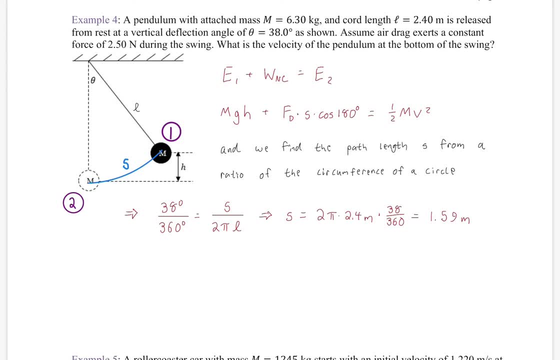 about circles. You can find that path really easily. This is a parabola or something You're not. you're not going to find the path very easily, and it ends up being 1.59 meters. So that's the path that friction acts over, because friction cares not about the vertical distance but about 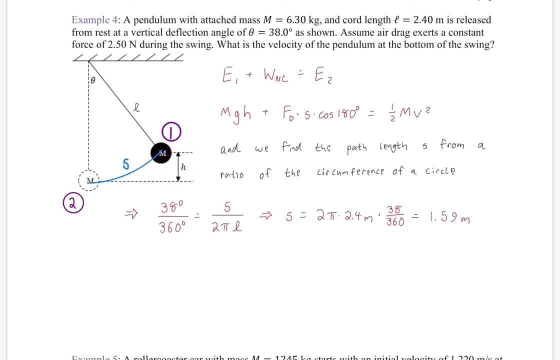 the overall path, Whereas, of course, gravity only cares about the vertical distance. All right, So then we're just going to solve for V, right? So there's basically our gravitational potential energy. This is the, you know, cause this, this, in other words this part, right here it would be. 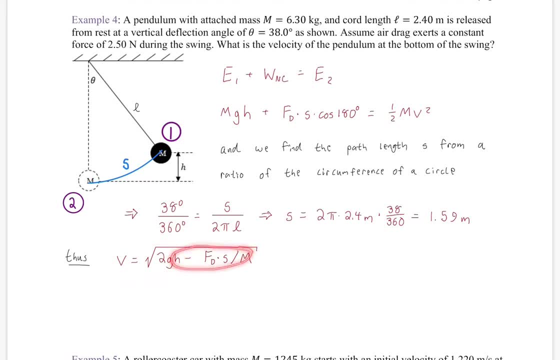 the answer if there was no friction. but see, then we have to subtract an extra value. if there's friction, making the V smaller than it would be otherwise, All right, Plug in our numbers and I'm replacing H with L times one minus cosine theta. Again, this is just from setting up a. 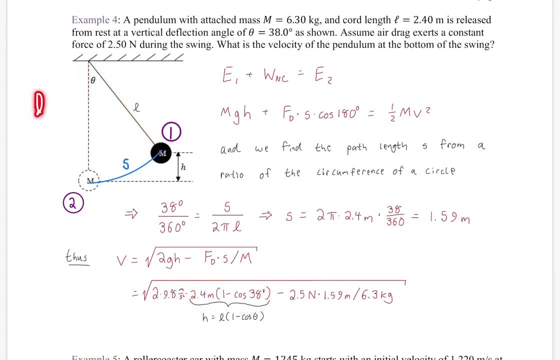 right triangle that looks like this, where the other side here is L minus H. Let's do this one more time. So this side is L minus H and this side is L. All right, There's our theta, And when I do that, I can find out that that's the relationship between H and L. 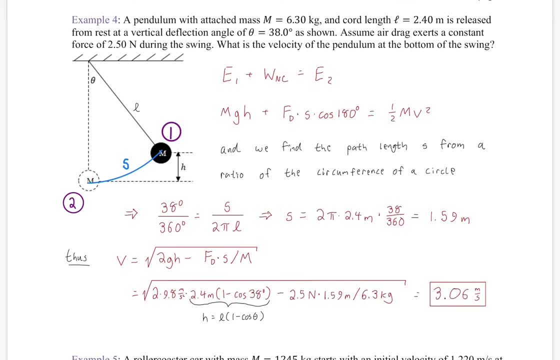 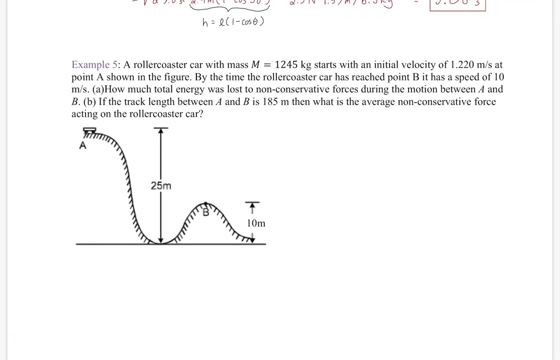 All right. And there we go, 3.06 meters per second, All right, Slower than it would be going otherwise, because air resistance, basically air friction, took away energy, Okay, Took away mechanical energy. All right, Let's do another one, A roller coaster with a mass of 1,245. 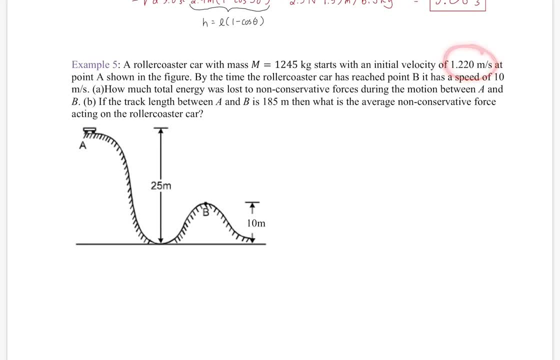 kilograms starts with an initial velocity at point A- 1.22 meters per second. All right. It's going to then go down, pick up speed, then go back up to that point, All right. But we find that the speed at point B is only 10 meters per second, That's. 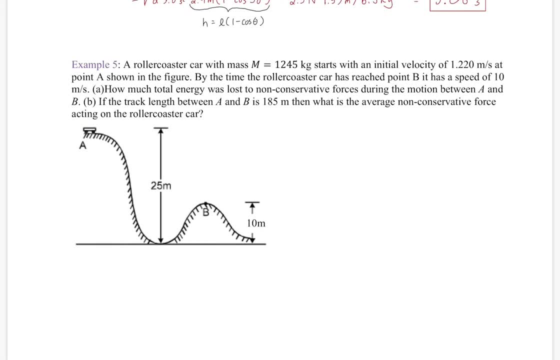 less than mechanical energy conservation would tell us. That means there had to be some non-conservative force, And I like this right, Because this is kind of a realistic thing. We could definitely take measurements at these two points and then find out: oh, there's some lost energy. and then 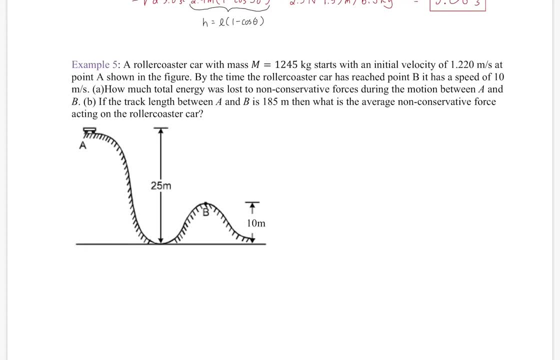 just account for that lost energy and say, oh, it's got to be a combination of friction and vibration and air resistance and sound energy, You know, all these things that are taking away from the perfect mechanical system. All right, So here we're. just we'll use the subscripts A and B, since they're already in the figure, rather than 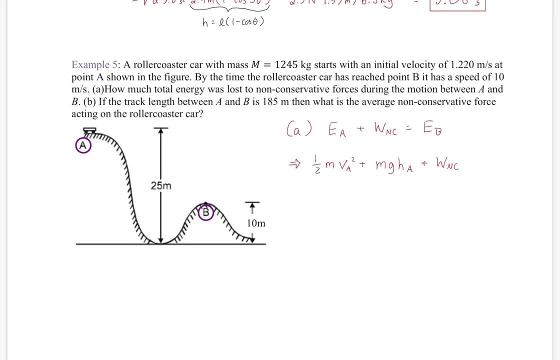 one and two. So EA plus work to non-conservative force equals EB. All right, Then we're going to just plug in our values here. Okay, This is all the left-hand side. Here's the left-hand side. We start with kinetic energy, We start with gravitational energy and we got our work from. 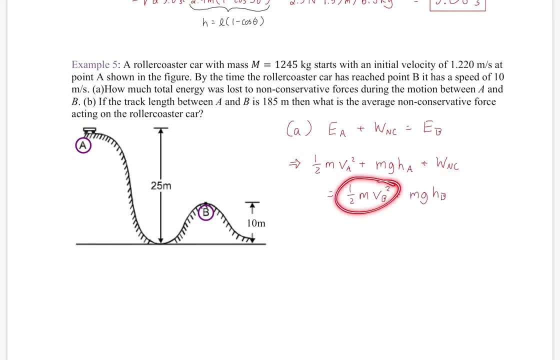 non-conservative forces, The right-hand side. we're going to have kinetic energy and gravitational energy as well. So there's actually a lot of non-zero terms here, Because at both A and B there was velocity and gravitational potential. All right, So then I'm 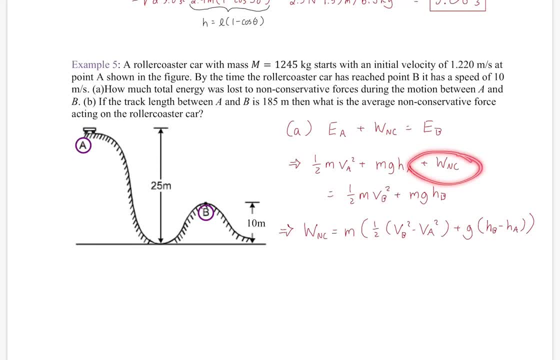 going to go ahead and solve for work by non-conservative forces. Again, that's important, that it's positive here. It would be negative if I considered. you know the directionality of the value at any given point, But you know when we actually solve for it here. 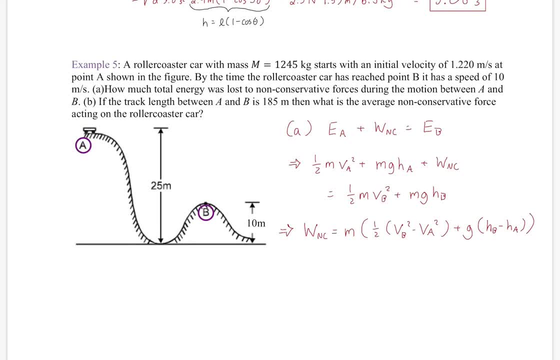 it's going to just naturally be negative because of where we put it. All right, All right In the conservation of energy equation, Okay, And then simplify it a bit, All right, I just combined all the like terms that I could and plugged in my numbers And I find that the work. 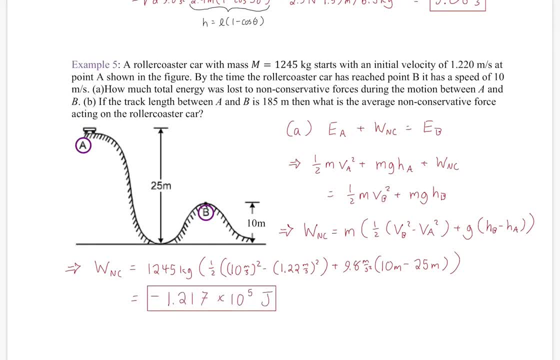 non-conservative forces is negative 121,000 joules. All right. It seems like I keep getting answers on the scale of a 10 to the 5, right, It's always 100,000 something. All right. So that's the. 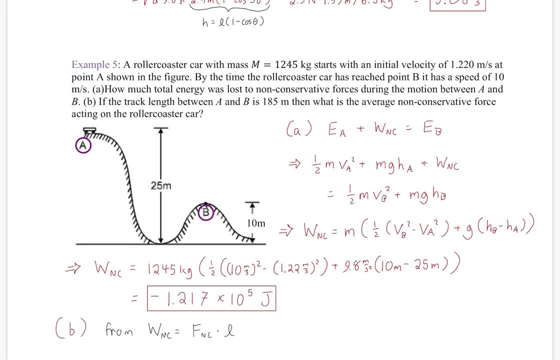 work done by non-conservative forces. Okay, And then I asked for the average non-conservative force. right, And this is kind of a combination. It's basically the average, because I said you know there'd probably be multiple forces contributing to this in the real world. So you, 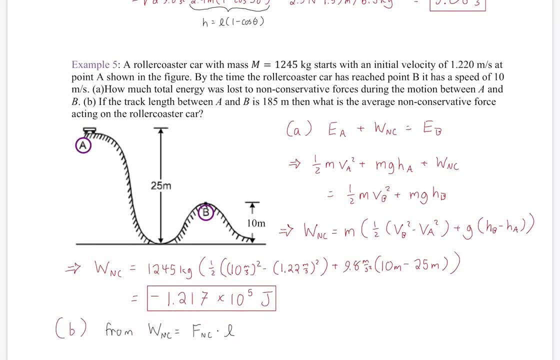 know the average non-conservative force. Okay, In that case it's just going to be FNC equals or WNC equals FNC times L, All right, And then we just solve. solve for that, Okay, All right. And 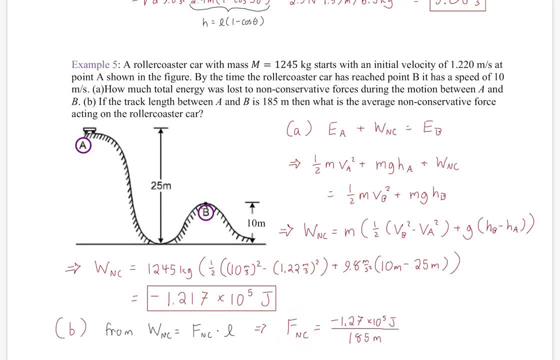 when we do, that force should be negative, because it should always be pointing in the negative direction relative to, basically, you know, positive velocity, And so then we have a force of negative 657.8 newtons. Okay, Cool, Pretty straightforward, but definitely just kind of. 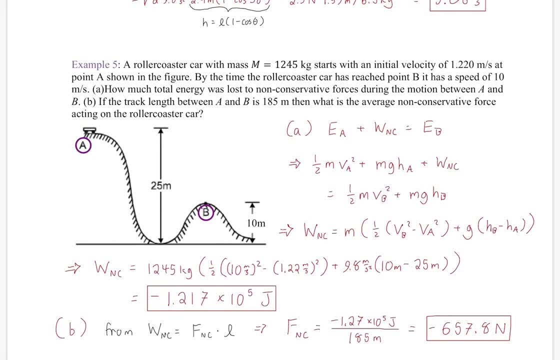 you know, this is such an iconic type of problem for non-conservative forces to do to have a coaster here, All right, And notice that I had to give you the path length And I couldn't like, have you know, just been clever and say, oh, it's a circle. 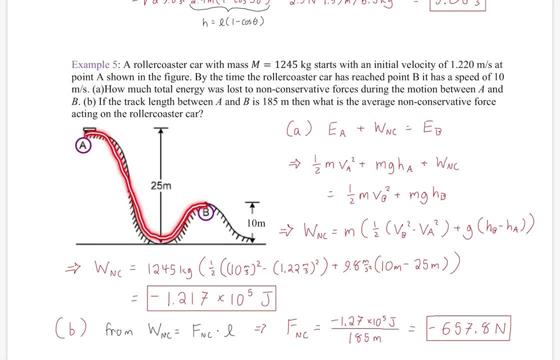 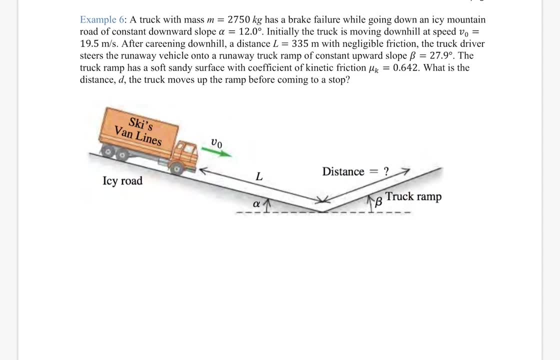 or something, because we have no idea what this curvature is. So you have to, it has to be exactly specified what that path length is, In this case, 185 meters. Okay, Last one, I would say okay. So this is. I'd mentioned this a minute ago as an example. it really highlights not being able to. 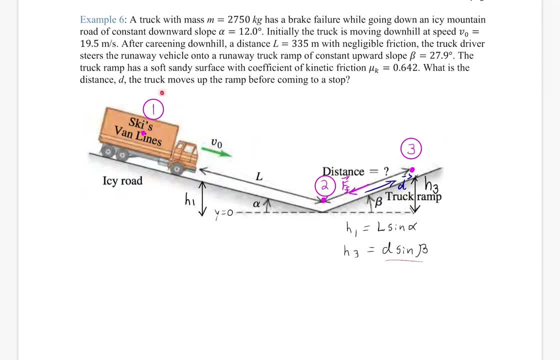 skip a step, unlike we could have with mechanical energy, because we have three points. We have point one, point two and point three. Between point one and point two is entirely mechanical. So there's friction between points, points one and point two. But then we're going to have some. 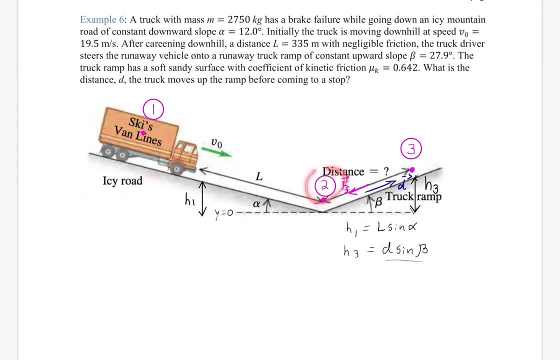 final velocity that we find based on conservation of mechanical energy at point two. But then, going up the ramp, there is friction. So then we have to define whatever energy is left over at point two, or is converted at point two really, and then find out what happens to it. to get up to point, 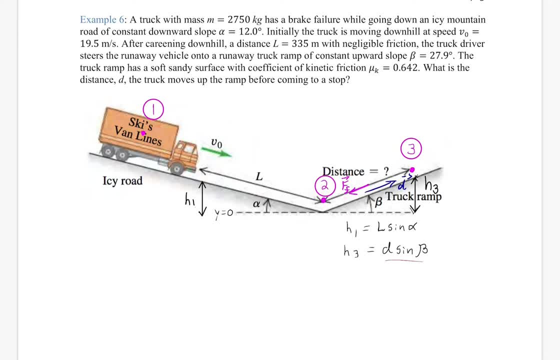 three, All right, So that's that's, that's the way we have to relate the our values in this problem, right? There's no, there's no kind of skipping ahead. Okay, I will mention, though, that, since these there's no curves here, this is we have, like you know, a 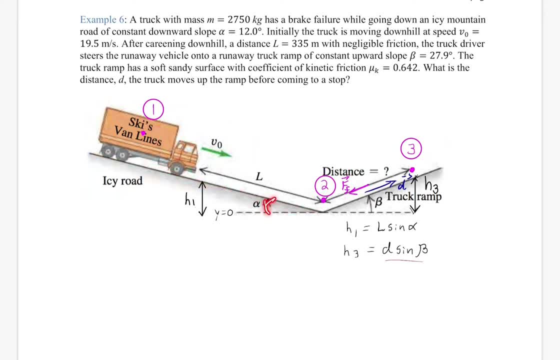 a uniform slope. you know, basically, a perfect ramp with a, with only one one slope, And then the same thing, a perfect triangular ramp on the other side. that we, you, can actually do this in this problem entirely with sum of forces. So, Newton's laws and kinematics, you can, you don't. 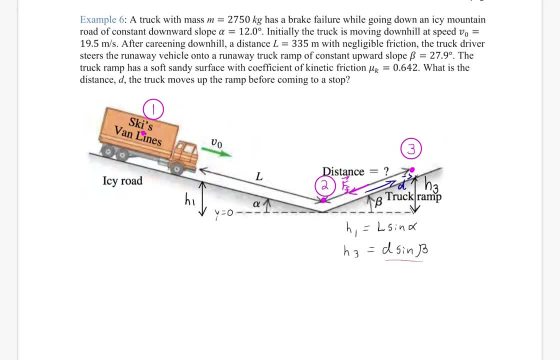 need energy for this problem. It's- I think it's easier with energy, but there's still. there's a lot of steps either way, But I've seen- I've seen students solve this problem entirely with Newton's laws and kinematics. All right, So let's just quickly run through the steps, All right? 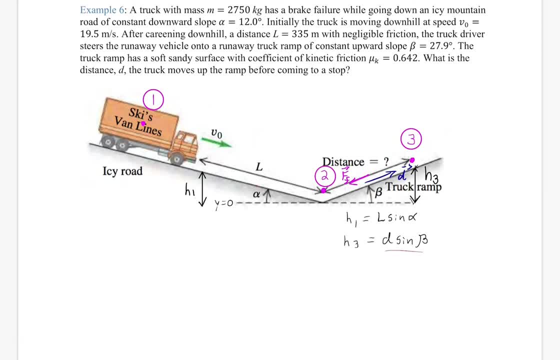 The problem? the problem consists of a truck. It's there was brake failure, So essentially it's just going to go down this hill at you know, and just pick up speed the whole time. The initial hill has an angle of 12 degrees, which is a pretty steep hill. It's got a length of, let's see, yeah. 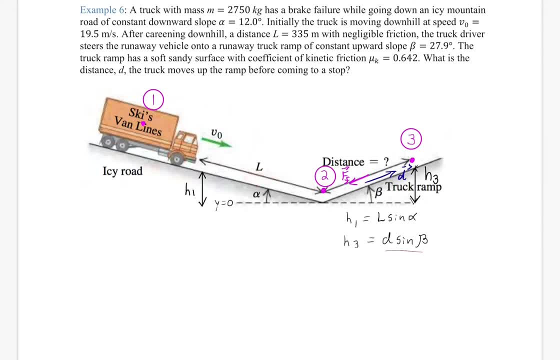 a distance of 335 meters. So that's our L. All right, We can use that to find H, because we weren't given H, we were given L. Negligible friction: The truck steers the runaway vehicle into the runaway truck ramp. You've probably seen those on freeways. All right, This the truck ramp. 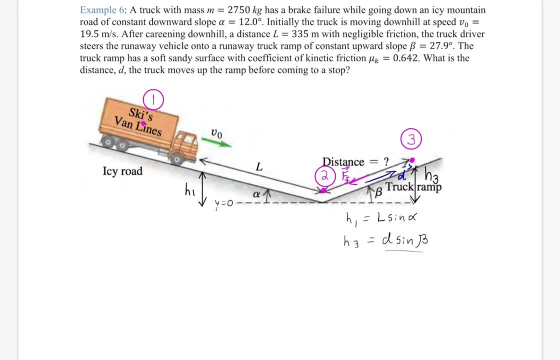 is very steep. It has a slope of 27.9 degrees. That's our beta slope. All right, And by the way, the truck started here, V naught at 19.5 meters per second. Obviously, it'll be going faster at. 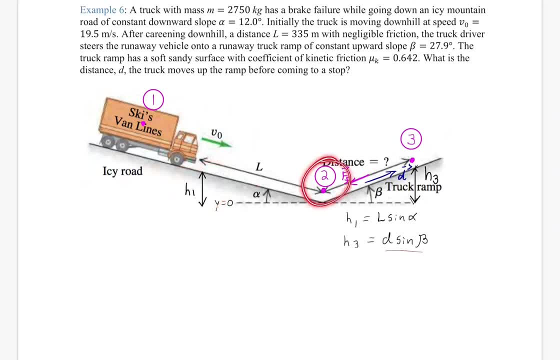 0.2, because the whatever gravitational potential energy it had will be converted to kinetic energy. All right, And then the truck ramp has a soft sandy surface, So it's got a lot of friction right- 0.642.. And what is the distance D The truck moves at the ramp before coming to a stop? 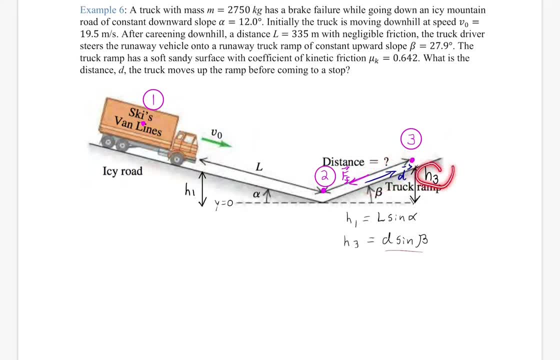 All right, So we're trying to solve for D and we'll, but we'll need H3 because we'll need to have some gravitational potential energy, Because when the truck goes from 0.2 to 0.3, you'll be losing mechanical energy to friction, basically converting it to heat, but also it's 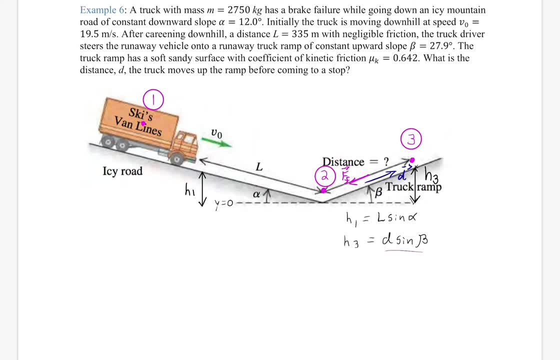 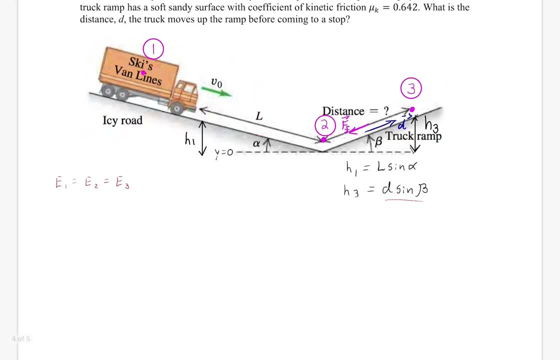 going to be losing kinetic energy to gravitational energy. right, That's the good thing about ramps pointing up. It means that friction. friction can do less work, Gravity can share the load, So we're going to have E1 equals E2 equals E3.. All right, In terms of energy, All right And okay. 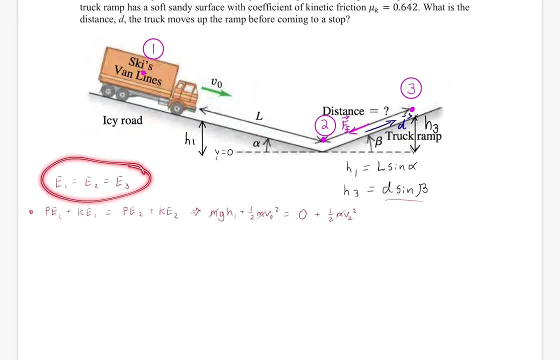 So we have potential energy plus kinetic energy, And when, when I write it this way, I'm you know, I'm acknowledging that this these are. this isn't mechanical energy, This is total energy. So there's obviously going to be between E2 and E3.. 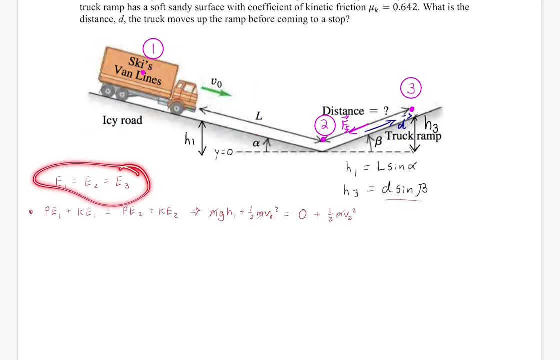 There's going to be plus work done by non-conservative forces, Okay, Which I kind of you know, kind of is a little vague in that, in that expression, but in general, of course, the energy is conserved, Okay, All right, And then. so this is just between one and. 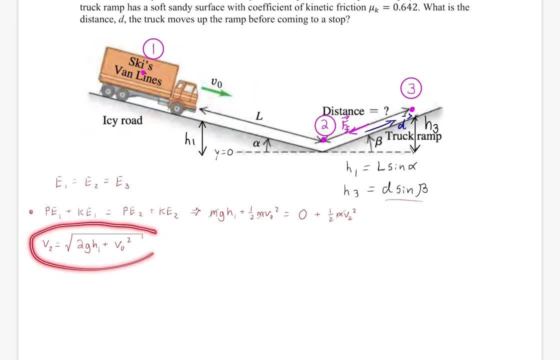 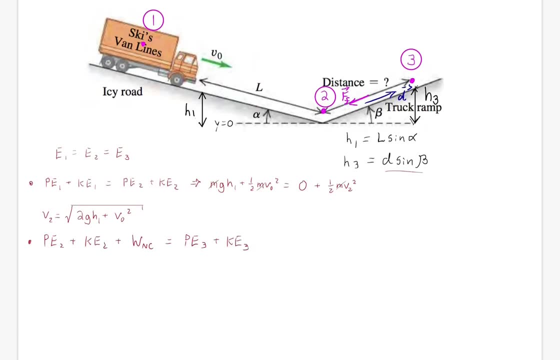 two. This is allow, just allow us all for B2.. I'm just going to express B2 symbolically in terms of height one and V naught Okay, And then we're going to go on to finding the energy conservation between E2 and E3. Here you can clearly see that I did put in the work by non-conservative forces. 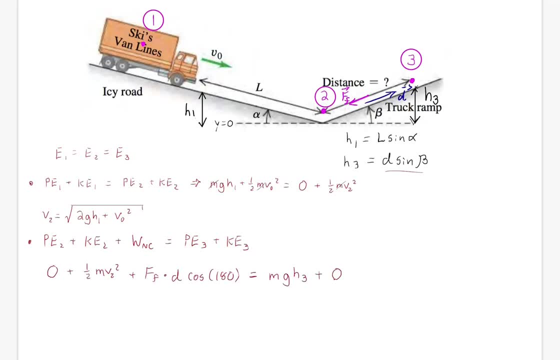 And here is the final energy at 0.3.. All right, So there we have. there's no potential energy at two because this is considered our Y equals zero point. All right, That that the you know kind of the bottom here, All right. 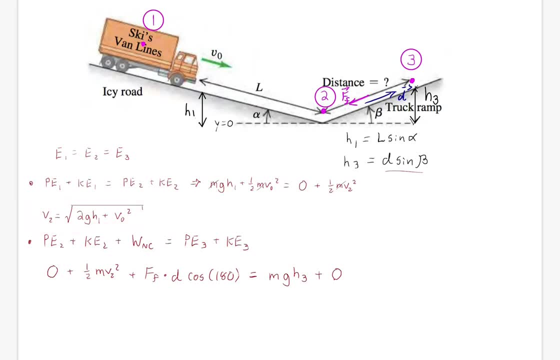 But there's definitely kinetic energy, V2.. We know what the value is And you can, you can find this numerically. I just wanted to keep it symbolic, All right. And then we have the, the work done by the friction right, Because characteristic cosine 180. And then the final energy is just: 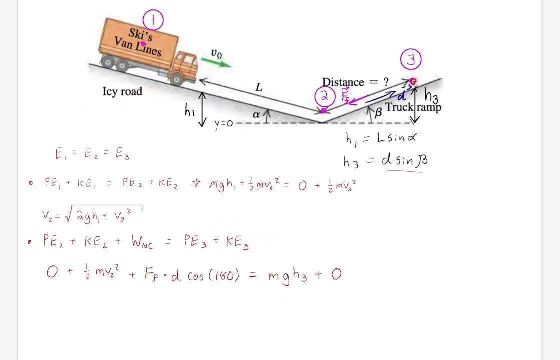 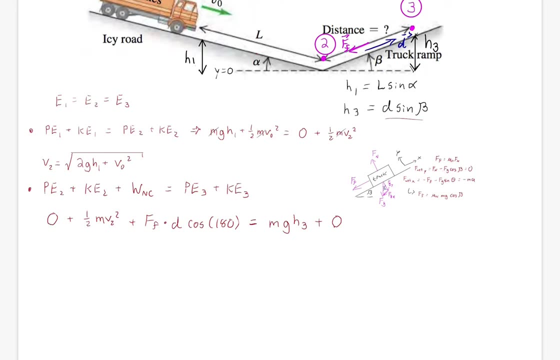 entirely gravitational, because there's no kinetic energy. at 0.3, because that's of course when the chart comes to rest. Okay, And then one thing I want to acknowledge is: what does the friction force look like? Because the friction force here is going. 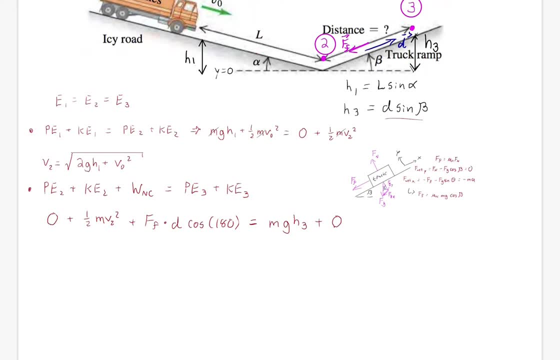 is going to be dependent on our sum of forces. We kind of maybe already recognize that. you know it's, of course it's mu K FN And since it's sloped, FN is just MG cosine data. It's just going to be the, the cosine component of the full gravitational force, And it's the cosine component. 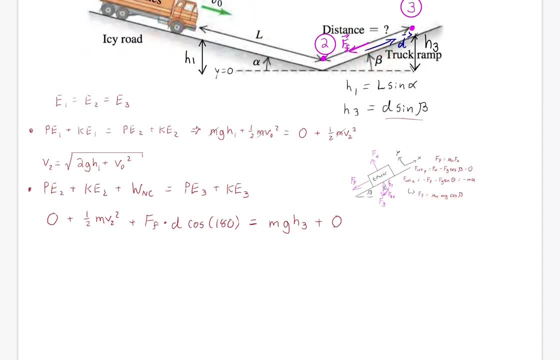 because their angle is measured relative to the horizontal. So maybe you just kind of have this memorized or used to it. but here's the full free body diagram to tell us where or what form the friction force takes. And that's friction force is going to show up right there. All right, So then 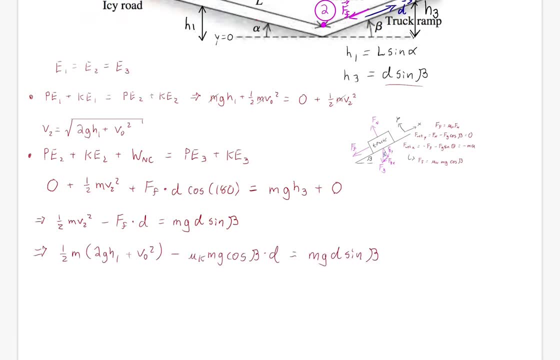 I'm going to go ahead and substitute that in here. I'm just cleaning things up a bit, All right. And then I substitute in the friction force in this step: right here, right here, All right. And then I also replaced H three with D sine, D sine beta. So we've got a cosine beta from the friction. We 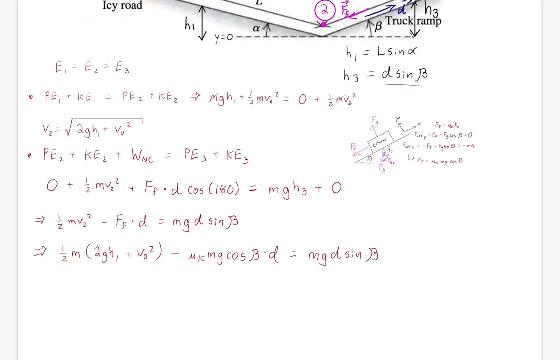 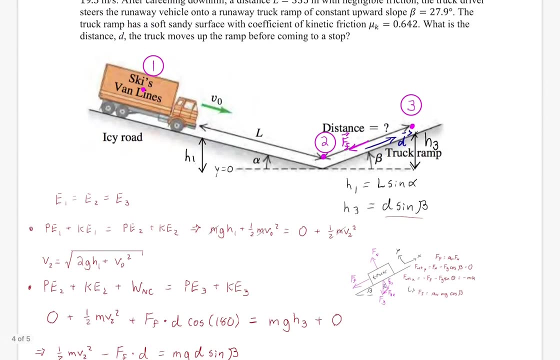 got a sine beta from the gravity. All right, We kind of bring it all together and then we're going to solve for H H three. Wait, is that what we're solving for? Yeah, Oh, D, we're solving for D actually, That's right. That's why we didn't leave it. leave it in terms of H three, And then we're. 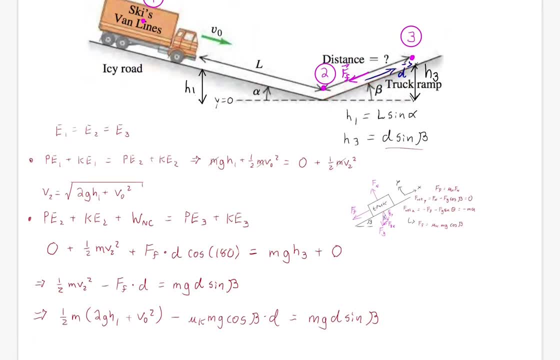 going to solve for H three, because we're solving for this distance. Basically, it tells us how long our runaway ramp has to be right. So we're going to solve for D. You notice that D shows up here. D shows up here. They're both as D's. There's no D squared or anything, because there's no spring. 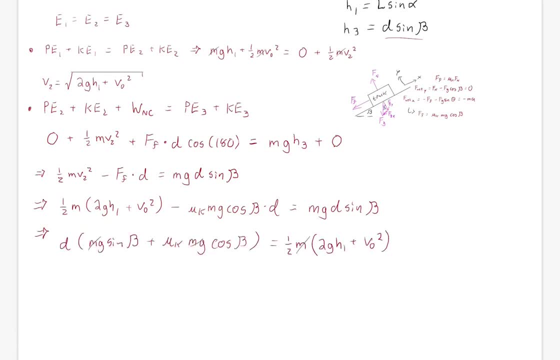 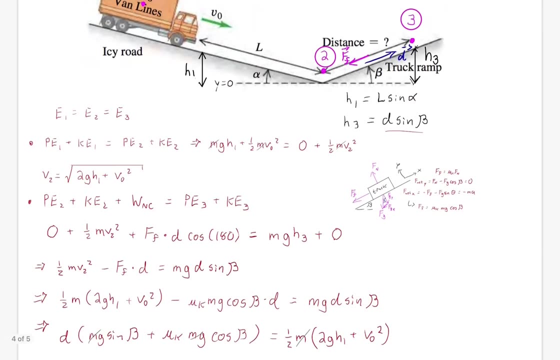 So it's simply a matter of finding that, solving for that D algebraically. Here I'm just doing some steps. The mass cancels out completely. Okay. So that's actually a nice thing here is because all the all the ramps are triangular. It's independent of the mass If we had a curved. 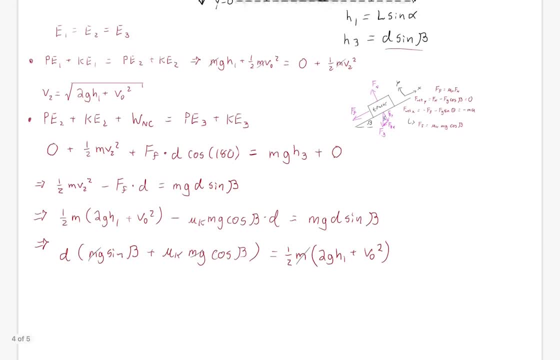 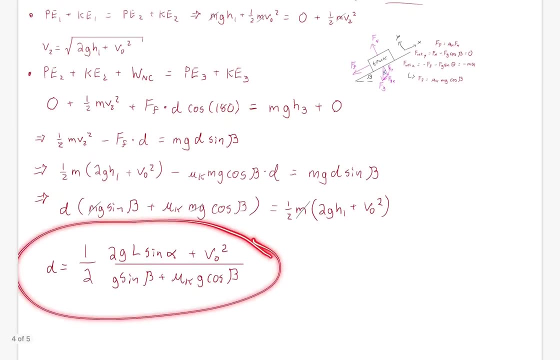 ramp, then the mass wouldn't cancel out. We saw that with the roller coaster. Okay, And then we have to have an average kind of friction force or average non-conservative force, And then we finally get this nice, nice expression right. It looks rather complicated. 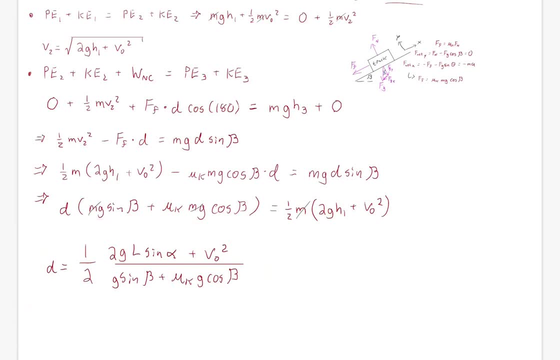 but it's. it did simplify quite a bit If you think about it. it's certainly that it's independent of mass, All right, And it's just. we got gravity in here. We've got gravity doesn't cancel because it doesn't show up in one of the terms in the kinetic energy term, You know. 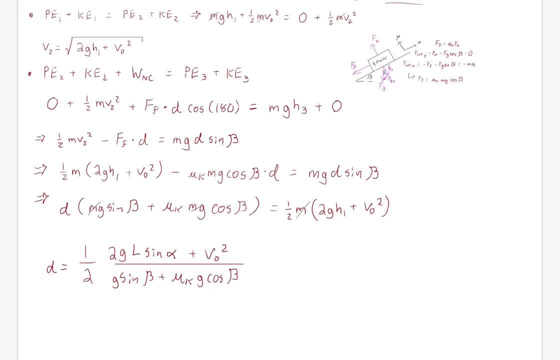 we've got the initial velocity. definitely, both the angles show up and only sign of the of the. the first angle shows up because there's no friction on that side, but it's both sign and cosine of the runaway ramp angle show up And then we've got the initial velocity.